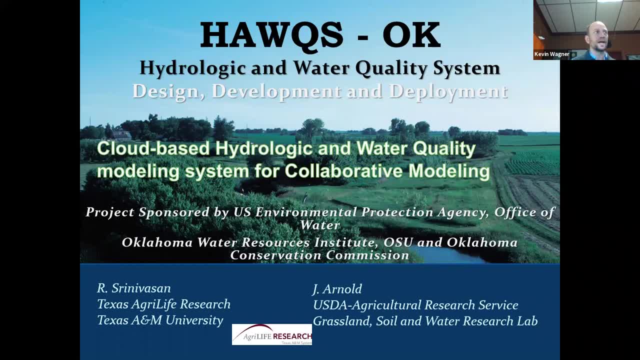 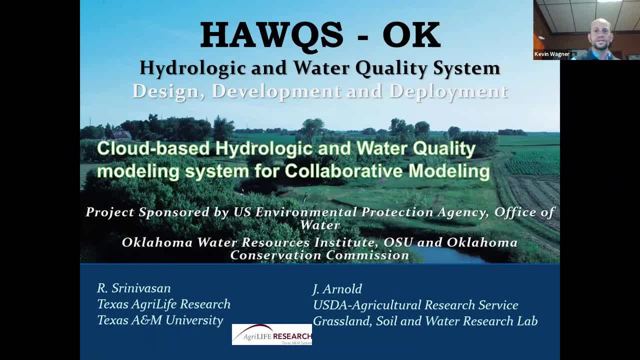 for their their work and their support of of this project, and then also certainly appreciate our partnership with Texas A&M University, want to note that we will be recording the session today. we're doing that so that we can make it available to others that aren't able to participate this afternoon, and 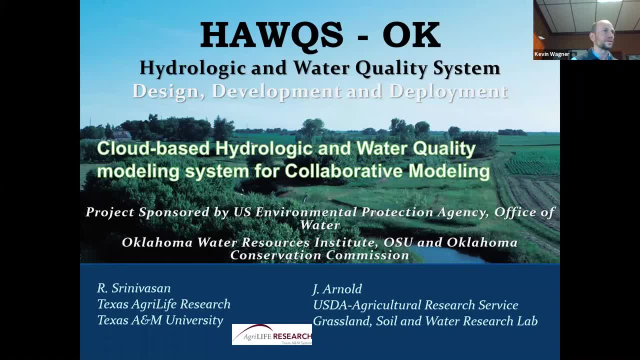 in the event that you want to go back and listen to parts of it as well, so it'll be available on our Water Center's website, which is waterokstateedu. I see everybody's microphones are muted, so please keep them muted during the presentation, but feel free to use the chat to ask questions as they arise at. 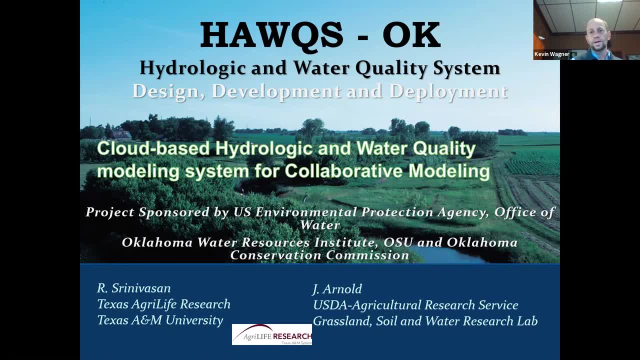 the end we'll have a Q&A session, and so we'll go through the chat and try to work through that as well. Thank you, So we'll go through those questions there as well, as you can certainly raise your hand at the end and and ask questions directly of Dr Srinivasan. So without 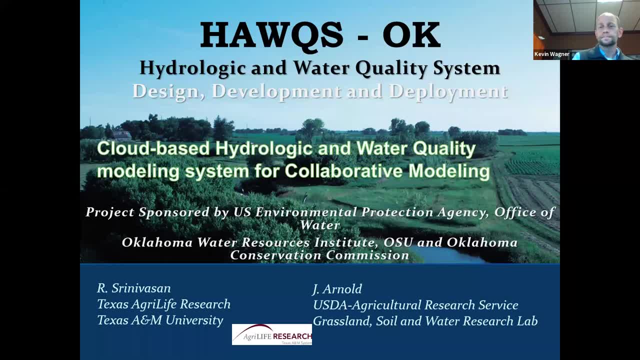 further ado, I'll turn it over to Dr Srinivasan. Thank you, Kevin. Can you all see my first slide and can you hear me well? Yes, Okay, so thanks for the nice introduction. Thank you, Thanks for having me. Thank you. 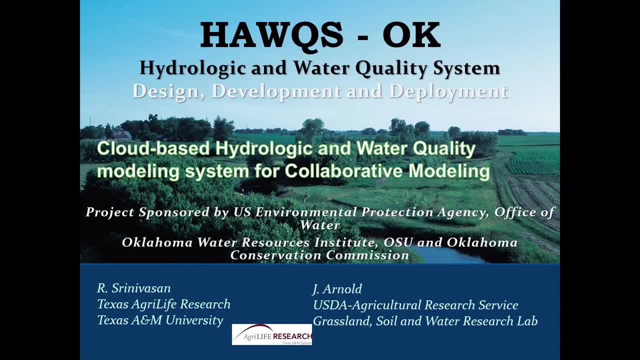 So the first question, Kevin, and like Kevin mentioned, HAWX, is a platform or a framework that integrates the model, especially the SWAT model, but in addition to that it also has got detailed database computer architecture that helps you to do over the cloud collaborative modeling so that multi-users and multi 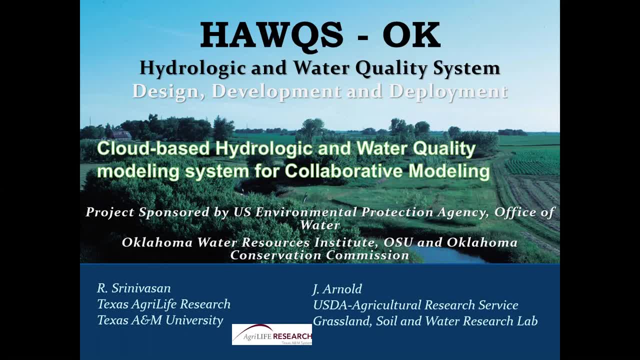 user discipline can work together in solving water quantity and quality problems. So I have acknowledged all those group here, especially the US EPA, who are the main sponsor of the, the original HAWX project, the National HAWX project, and certainly it won't be possible without the. 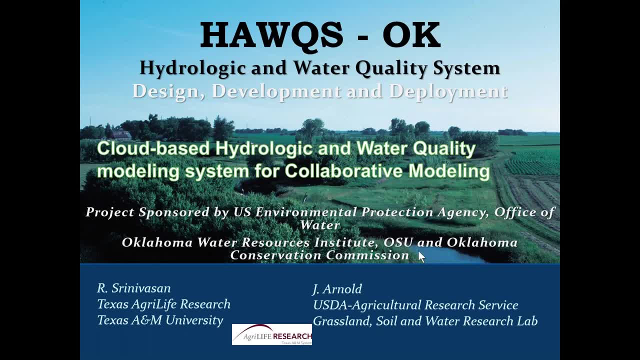 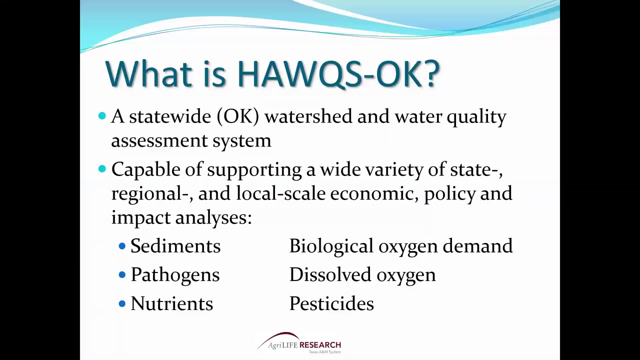 Kevin's group, as well as the Oklahoma Conservation Commission, in developing Oklahoma specific version of HAWX, with more detailed input and the calibration and so on which I'll talk a little bit later. Okay, so with that. so what is HAWX? HAWX is a statewide watershed and water quality modeling. 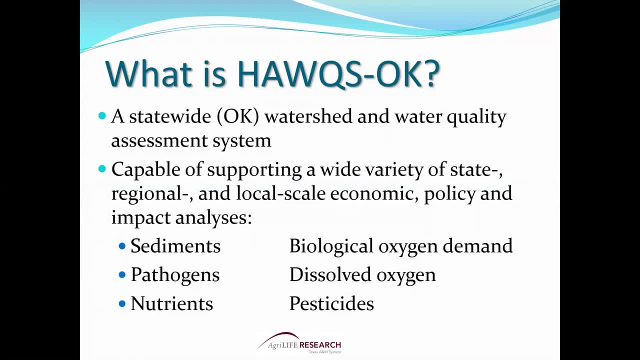 system and it's capable of supporting wide variety of state, regional and local scale economic policy, as well as impact analysis, like TMD and other projects. So I'm going to turn it over to Kevin. Yes, so let's to the current state of the topic. This is the water quality assessment model. 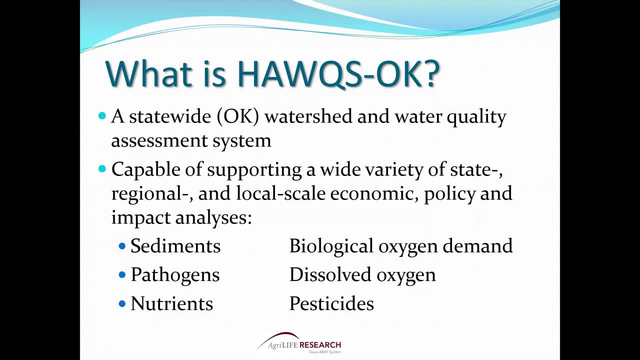 For both HAWX and theater and laut. I will start with the HAWX system. Just to start with, we have a nuclear level, a nuclear� system, and in order to do that we have to have emergency water quality standards. So you can see here that the water quality settings in HAWX are not exactly the same as in the water quality assessment model. 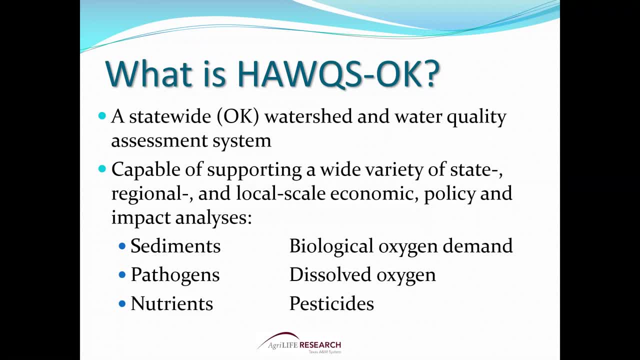 but we are able to support yourself. So let's start with the HAWX system and the water quality assessment model. you, as a user, can bring your own input and you're able to run using an existing HAWX system. So it is a nice way of using existing knowledge and adding your own specific knowledge to model a watershed. 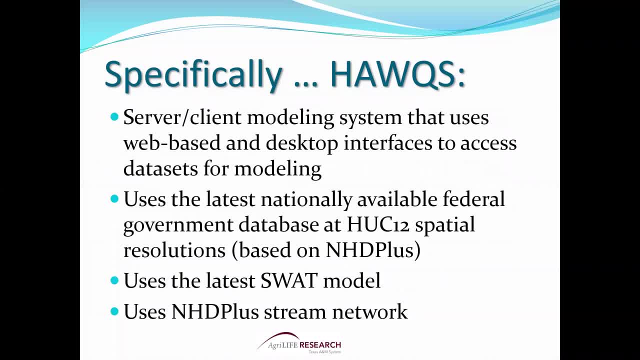 In more specific terms, HAWX is a client server modeling system, meaning it's a web-based, cloud-based technology. You can use it with no GIS experience. You don't have to have any powerful computing systems, You don't have to have any knowledge specifically about the data, how it's integrated and things like that actually. 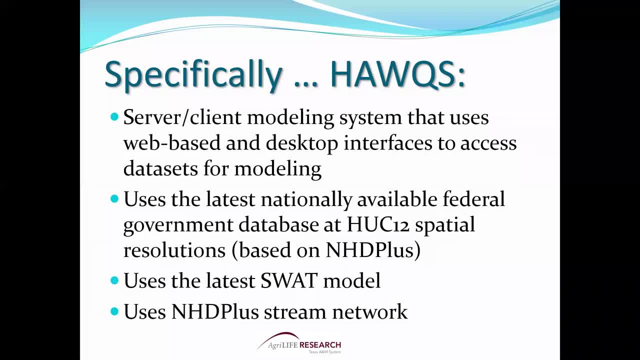 So a lot of those data are then behind the scene on the server side, So you as a user may not have to worry about it. So you can even use your, say, smartphone like iPhone Or iPad or any kind of tablet system or a desktop system. 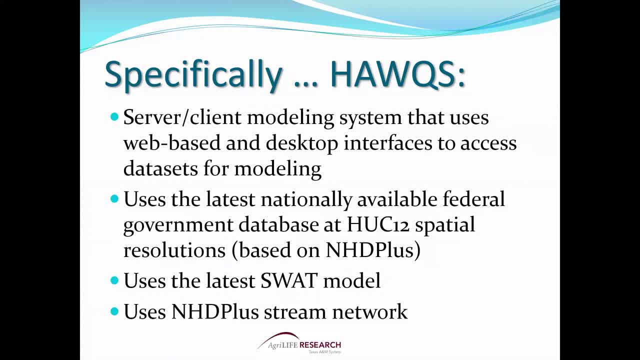 As long as you have an internet connection, you can connect to the server And you don't have to stay unconnected. actually, You can submit your job, walk away and you can come back and continue. So I'll be doing a demo, a live demo, at the end of the presentation to highlight the features. 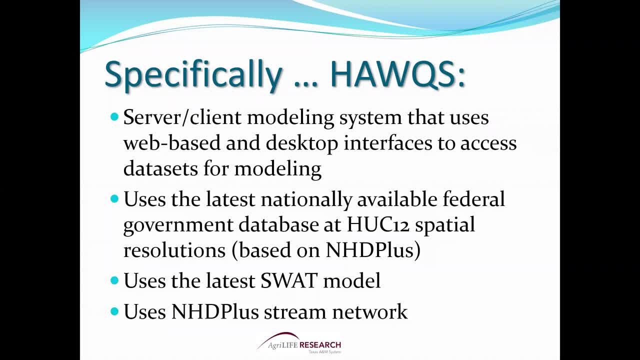 So it is using the latest both nationally and Oklahoma specific data set for the HUC-12 spatial resolution And we are using the NHDPlus for the stream network, more detailed stream network and uses the latest SWAT model And it uses all publicly available data that can help to set up the model or set up the HUC system. 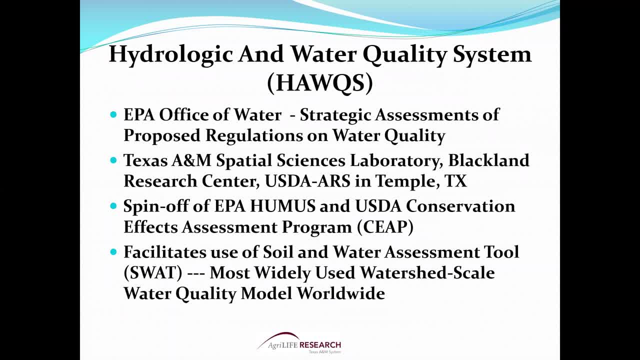 This has been going on for quite some time. The Office of Water- EPA Office of Water- helped us to develop the HUC system, And Texas A&M and USDA ARS are integral part of that. But the national work of verifying and validating and improving the SWAT model came from various other national projects. 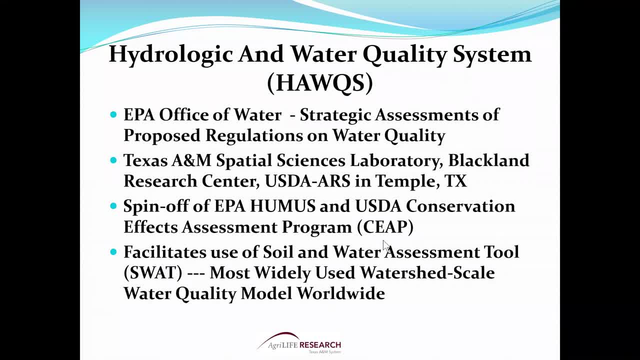 such as the HUMUS SEEP. These are all some of the projects that have been going on in decades at Temple Texas. Okay, And some of you are already familiar, SWAT is a well-known model around the world used for water quantity and water quality assessment. 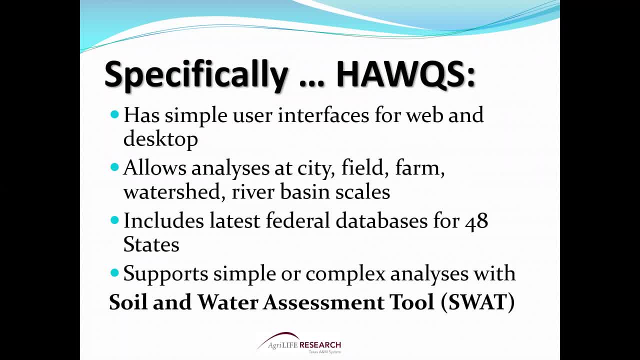 HOCS has got a very simple GIS interface, just like Google Earth or Google Map, where you can just simple point and click and you're able to develop your own watershed at the HUC-12 specific And you could also analyze the data at the form or field level. 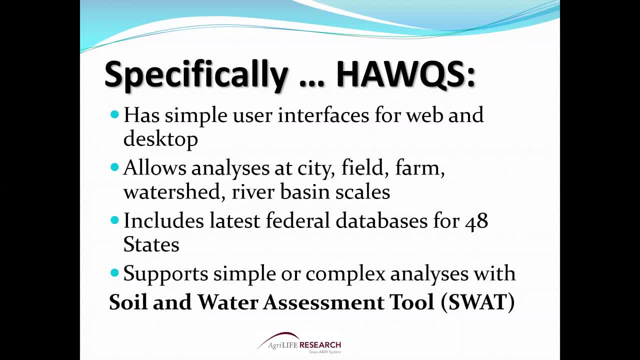 by examining individual hydrological response units in modeling any watershed or in any field or forms. Okay, It supports all the way from very simple to complex analysis. What I mean by here is: HOCS is going to provide you a framework to do: set up your model, run the system, do the scenario analysis. 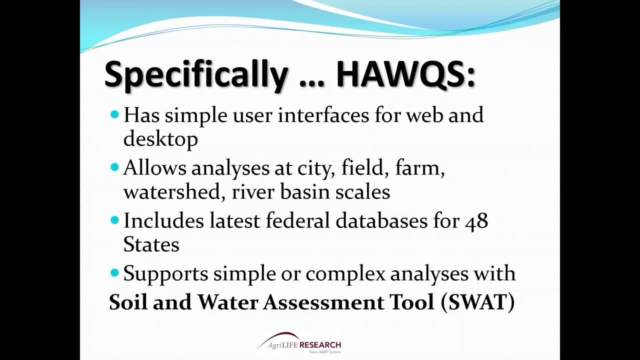 compare the scenarios, Like visualization and statistics and so on and so forth, But HOCS is not going to mimic what SWAT can do on its own, like a desktop system, for example. So HOCS allows you to do almost most of your functions, or most of your analysis, on the server side. 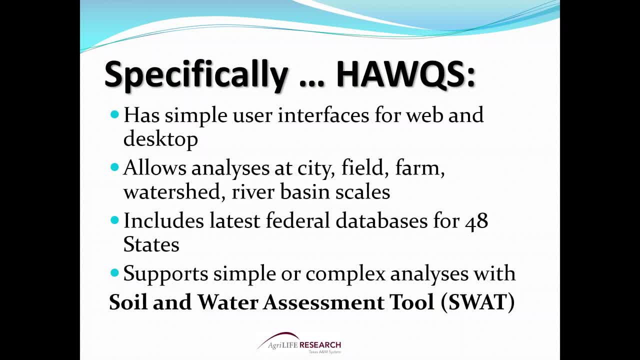 But as a researcher, you may want to explore more things. that's not available in the HOCS system. So the HOCS allows you to download the entire data and be able to do much more complex or comprehensive analysis at your local desktop. 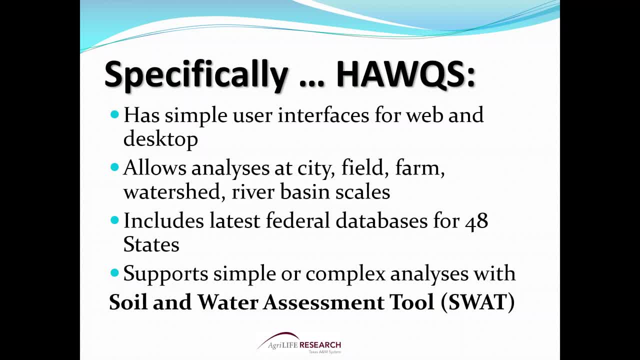 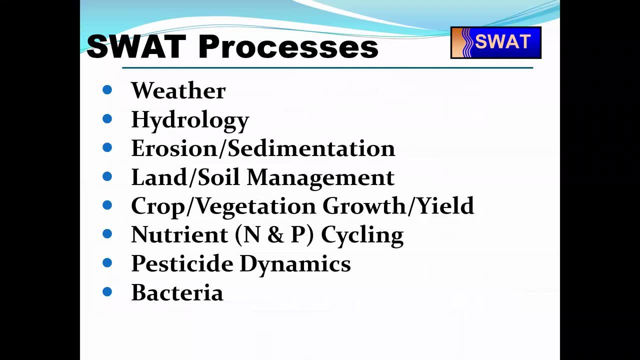 So the data sets is available both online and offline so that you could build a model and analyze that model inputs and outputs without needing to have additional computing or additional GIS software. For those of you who may not be familiar with SWAT model itself, I have a few slides to go through that very quickly. 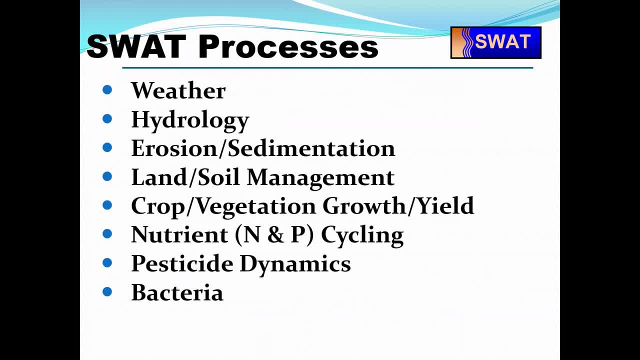 And I know some of it may be repetitive for some of you. Please bear with me. So SWAT has got various major landscape processes. The main strength of the SWAT is the landscape processes where the weather drives, your hydrology, your comprehensive hydrology, which you will see in the next slide. 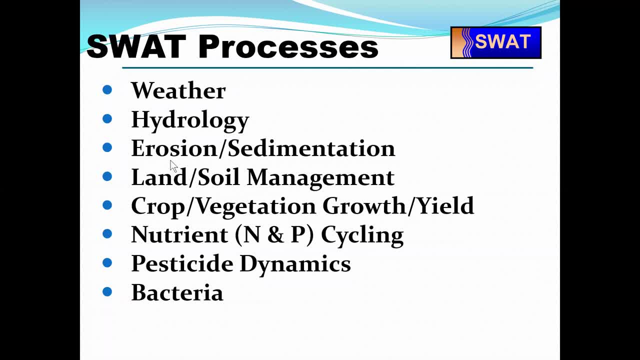 And erosion and sediment process, both landscape and landscape processes. The land and soil management in terms of crop management, vegetation management or looking at tillage, pesticide, fertilizer and so on and so forth. And the nutrient cycling, including carbon and bacteria, is included in the model. 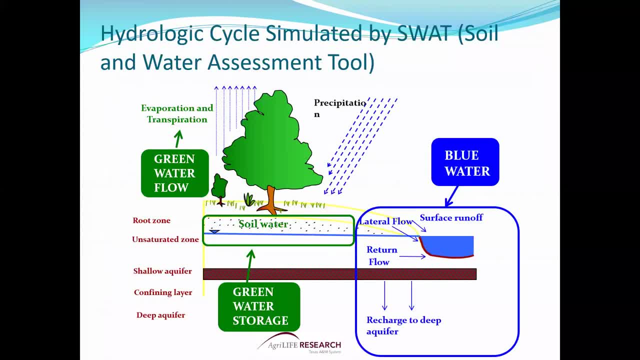 So this gives you a comprehensive overview of how SWAT deals with soil. So this gives you a comprehensive overview of how SWAT deals with soil. So this gives you a comprehensive overview of how SWAT deals with soil. And then there's several other hydrological components. 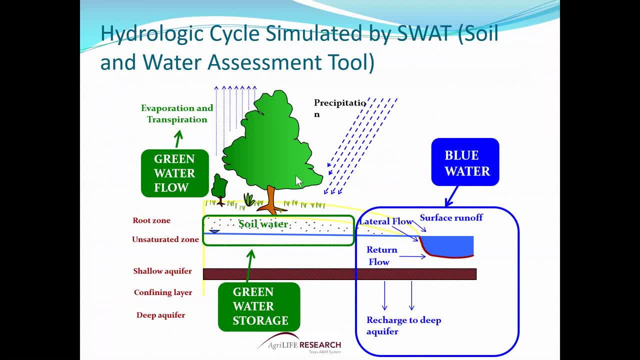 And in rainfall is the only input here. then you need to tell what vegetation is growing on this soil, and the SWAT model will give you outputs such as: how much is evapotranspiration, for example, how much is the runoff, how much is the lateral flow, how much is the return flow. 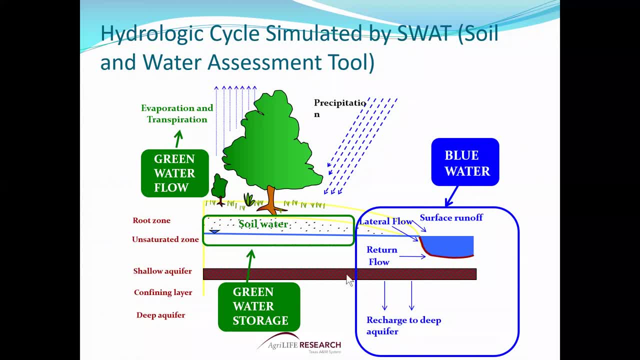 how much is retouched to the groundwater, and so on and so forth. Okay, so it has got sets of equations that govern each of these processes. Okay so, it has got sets of equations that govern each of these processes and you'll be able to get output from each of the intermediate variables as well as the final variables. 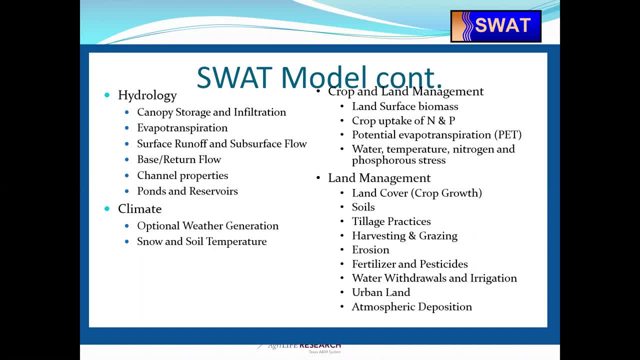 Okay, Again, I'm not planning to go through every one of them, Just to give you. on the hydrology, we do take into consideration of the canopy storage and infiltration evapotranspiration. We have three different sub-modules within evapotranspiration to use. 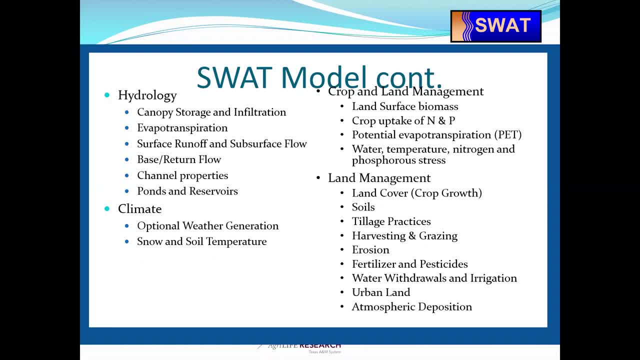 such as Penman, Hargrave or Priestley-Taylor method and so on. It has got subsurface flow and surface runoff, base flow and return flow, channel characteristics like channel loss, channel evaporation, Ponds and reservoirs also can be modeled. 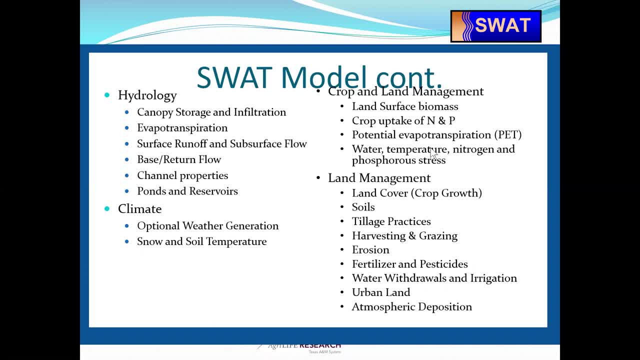 So one of the major strengths of the SWAT is the crop or vegetation that you can simulate and able to verify and validate crop biomass or crop yield, and thereby you are able to validate the nitrogen and phosphorus uptake by the plant and the nitrogen-water-phosphorus balance in the soil and so on. 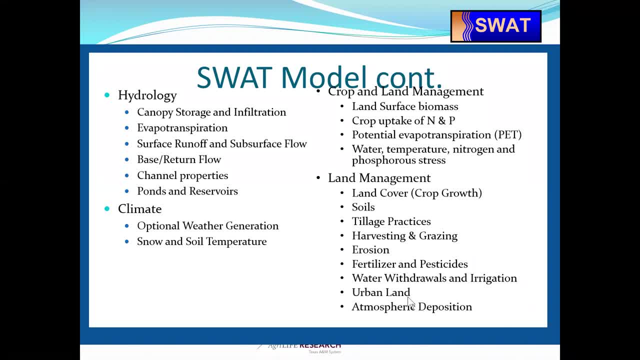 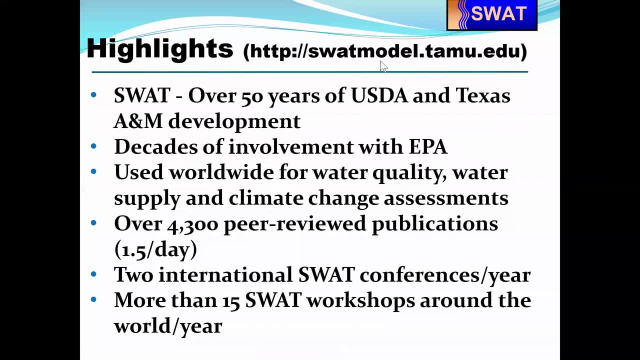 And also it has got a very detailed land management. just as listed here, SWAT has been in development. If you want to know more about the SWAT itself, you can go to the swatmodeltamuedu website. It's in development for well over 50 years and it's been well adapted. 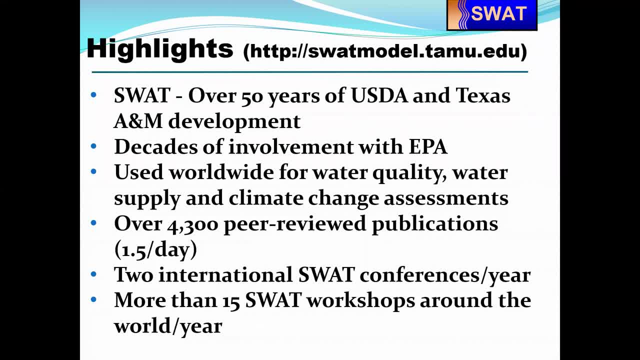 worldwide with many, many, many projects and verified and validated. We have more than 4,300 peer-reviewed publications and our average publication per year is about 500, which is about 1.5 per day. is the number of publications using SWAT model around the world actually? 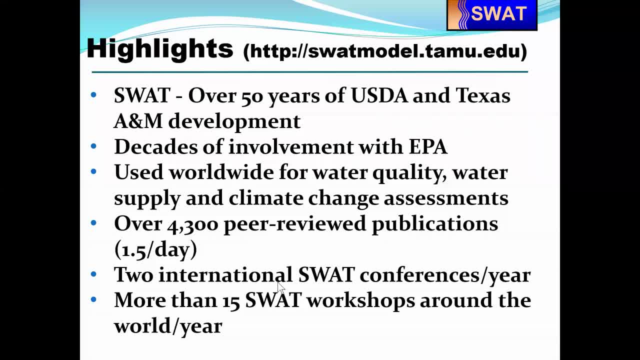 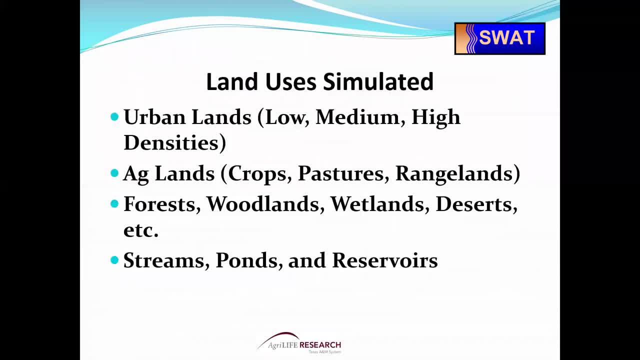 We do conduct a lot of conferences and workshops if you are interested in getting in more detail. So specifically in the Oklahoma hawks we are simulating all the urban landscapes, the ag lands. that includes the managed and unmanaged pasture and rangelands. 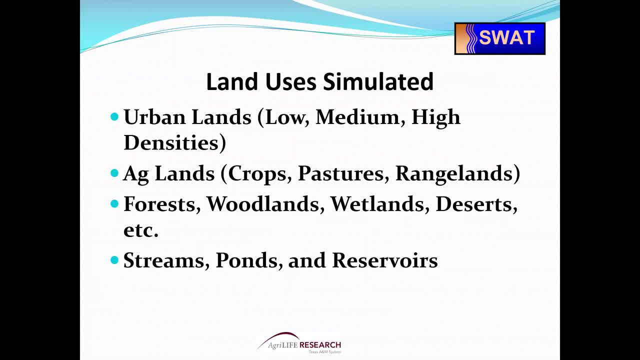 forest, woody biomass, as well as wetlands and any kind of barren land and so on. And in the stream processes it takes into account of all the stream, channel morphology, geomorphology, the ponds, reservoirs and wetlands. our model: 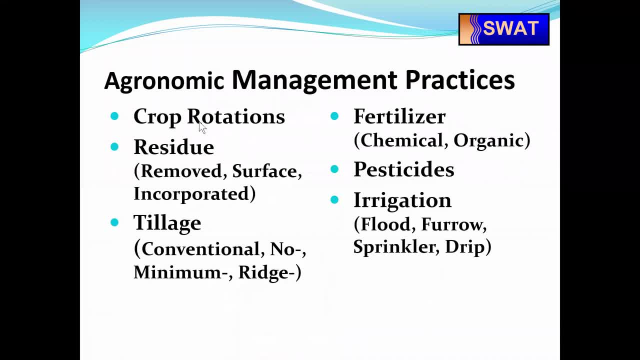 In the agronomic practices. we're looking at the crop rotations. We are using the crop data layer of 2016,, 17, and 18 to look at the crop rotations, and those crop rotations are included: The crop residues, the tillage, the fertilizer. 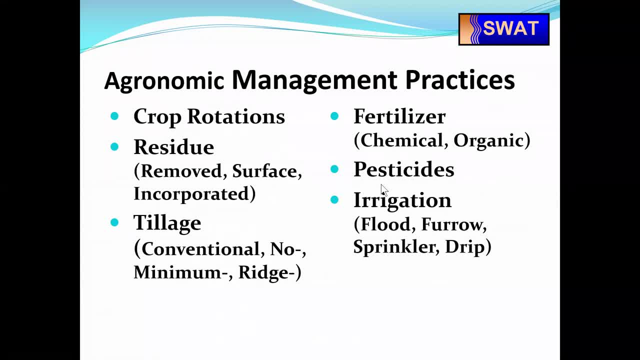 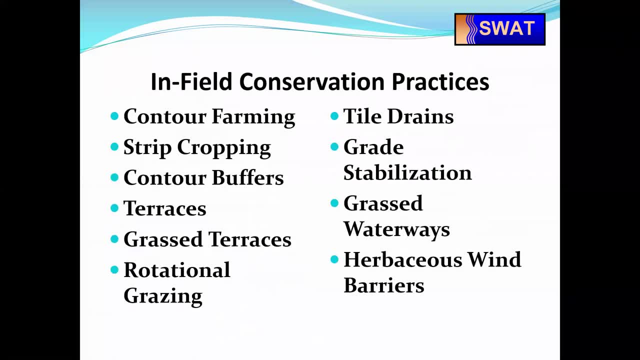 the pesticide is capable of inputting pesticide, but we don't have specific inputs yet And if there are irrigation, we do take into consideration of irrigation And in field conservation practices you can simulate various tillage practices, tile rains- if you have the tile rains, grazing management. 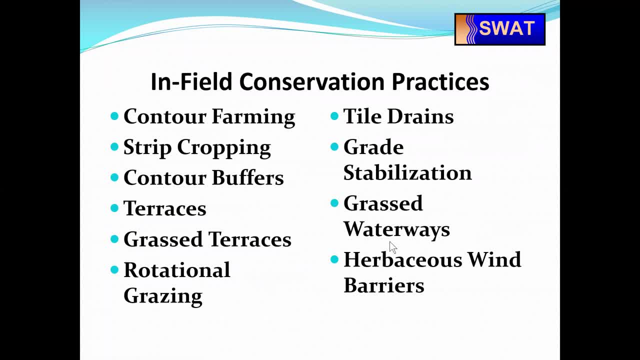 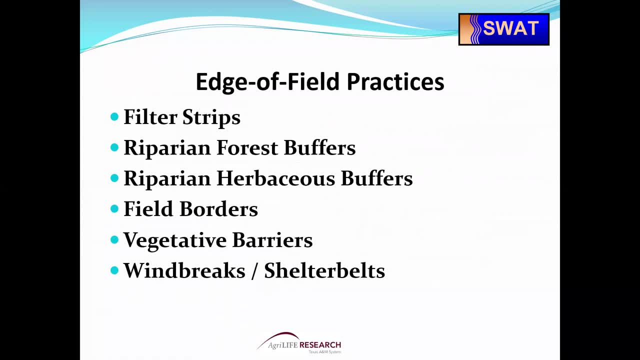 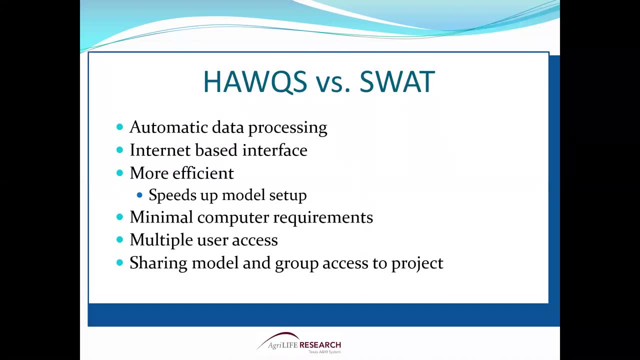 or grass, waterways and so on. We can also do the edge of the field buffer practices like filters or riparians and field borders And so on and so forth. So what is HAWX and what is SWAT actually? HAWX provides you an automated way to process the SWAT inputs. 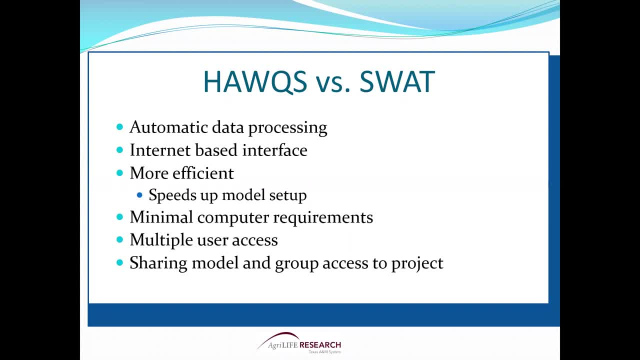 based on internet-based interface, meaning a web-based interface. It's most efficient. When I show the demo, you'll see within a few minutes you'll be able to set up a watershed anywhere within the state of Oklahoma And you need only a minimal computing requirement. 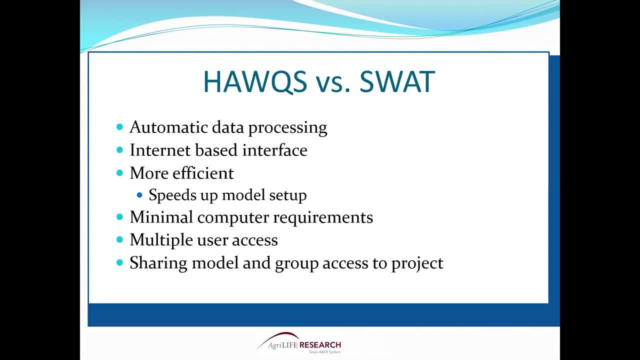 You don't have to have a very heavy equipment and you don't need to worry about having all the software, license and everything. Everything what you'll be using is public domain-based information And you can have multiple users accessing simultaneously the HAWX system. 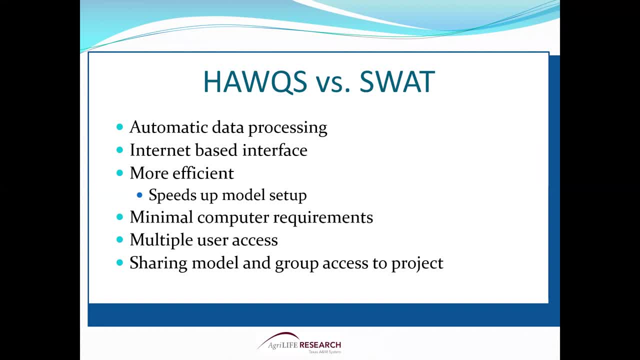 so you're not worried about having only one user access or limited user access And, most importantly, in the most updated HAWX system we do have sharing of models. So if you have a hydrologist who could be verifying and developing a model for hydrology, 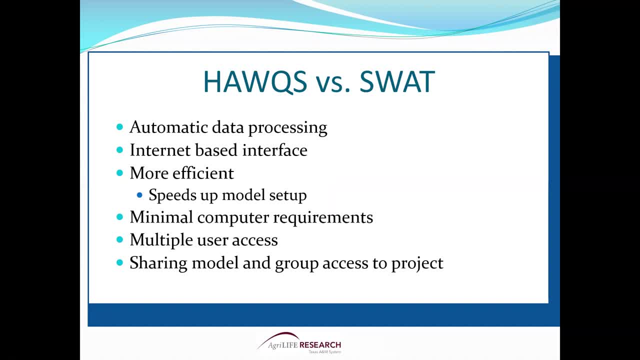 then there could be a water quality specialist or an agronomist or a soil scientist can look at the water quality aspects. because SWAT deals with multidimensional or multidiscipline fields of expertise, So you could be working in a collaborative so you can set up a project and share that within your group. 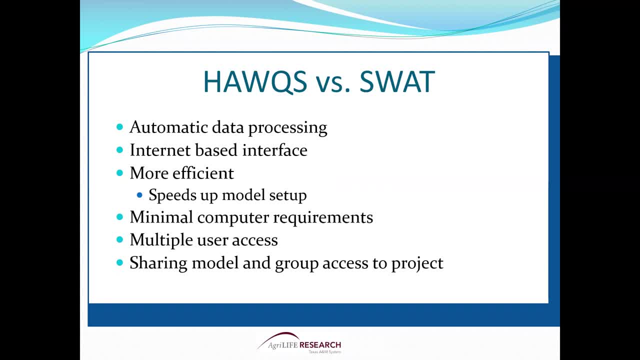 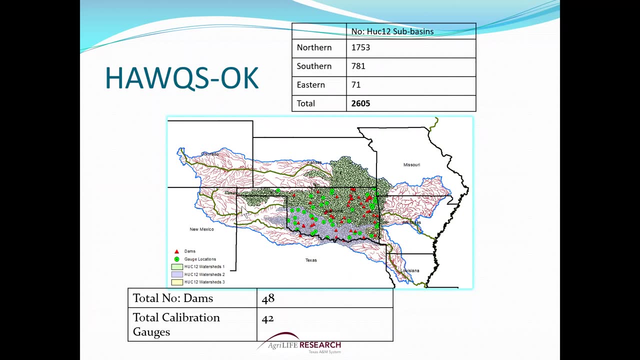 and they all can have access to the same model while they are developing their scenarios or checking the model results, and so on and so forth. So this is what will be set up for the HAWX Oklahoma. We have about three segments here, actually. 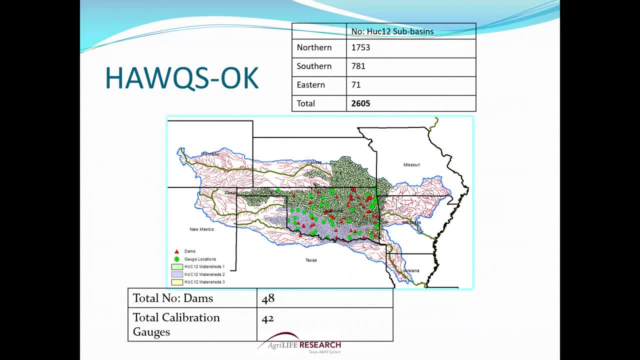 I don't know if you're able to see them very clearly. This region here, which is mostly the Arkansas River, there are about 1,753 HAWX-12 sub-watersheds, The southern one which is mostly bordering. 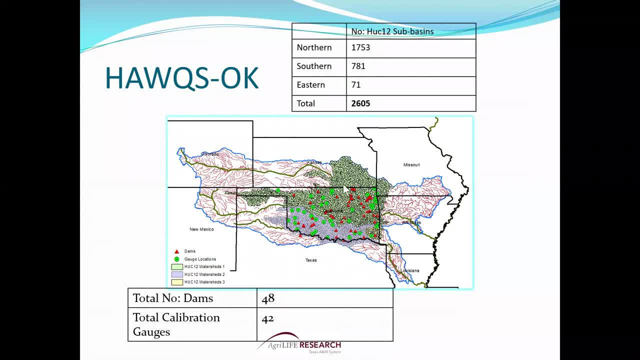 between Oklahoma and Texas. that's about 781 HAWX-12s here And there are a few that's originating right at the eastern end of Oklahoma. that are about 71 of them. In total, there are about 2,600 HAWX-12 watersheds. 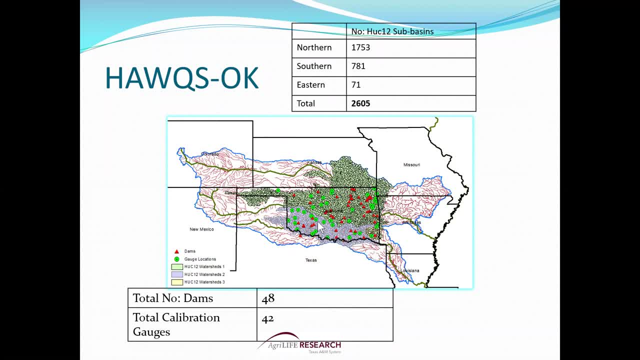 that comprises the whole state of Oklahoma, And the green dots are the gauge locations where we have planned to do calibration for hydrology at a monthly scale, And that calibrated model setup is what's available so that anywhere when you run the model, you have a calibrated model for hydrology is set up. 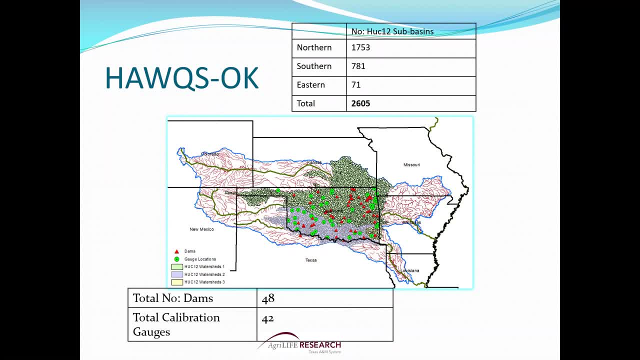 before you can even start any scenarios and things of that nature. And the red triangles are the existing major dams that will be incorporated in the system also, So there are about 48 major dams and about 42 calibration sites we are planning at this time. 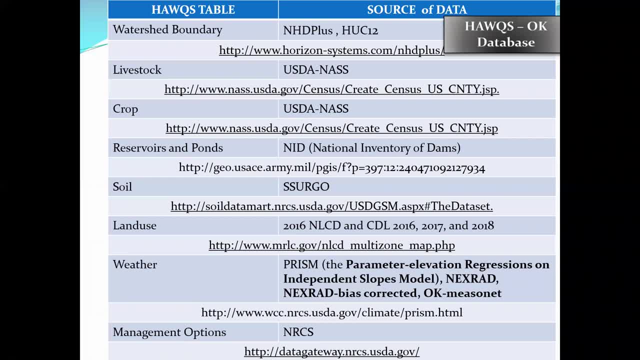 Here are the list of data sets. I don't expect you to go through them. The major differences here: I wanted to talk about the national losses. here is the crop data layer is based on the CDL and NLCD 2016.. And the soil is based on Sergo soils map. 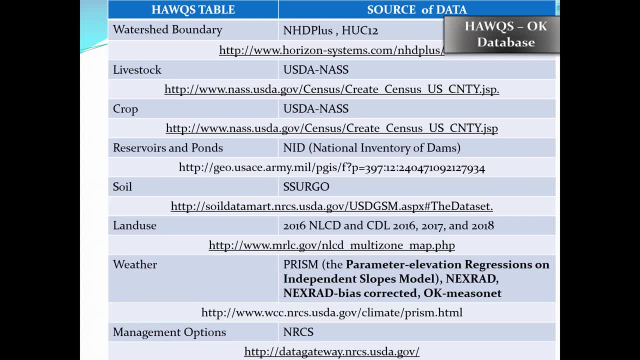 whereas national is Statsco. And, of course, here is the land use NLCD 2016 and the CDL 2016 and Sergo, And we will have four sources of weather data that one can use to set up the model actually, 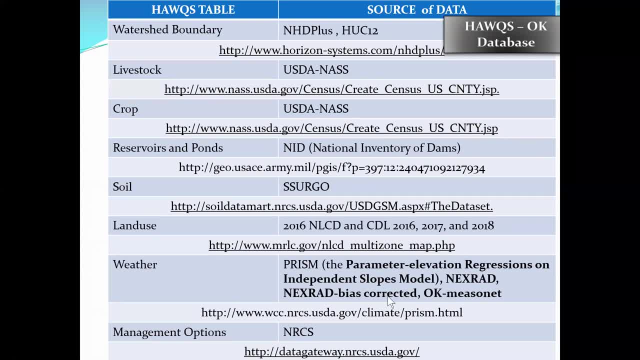 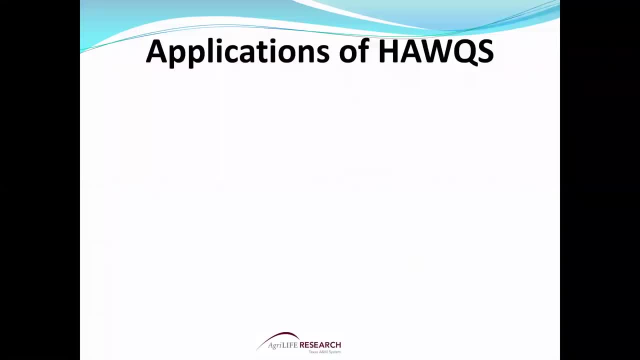 The PRISM, the NEXTRAD, the NEXTRAD bias corrector, as well as Oklahoma Mesonet data set. So what can you use the HOCS for? HOCS could be used to evaluate the land management, crop management, such as fertilizer tillage. 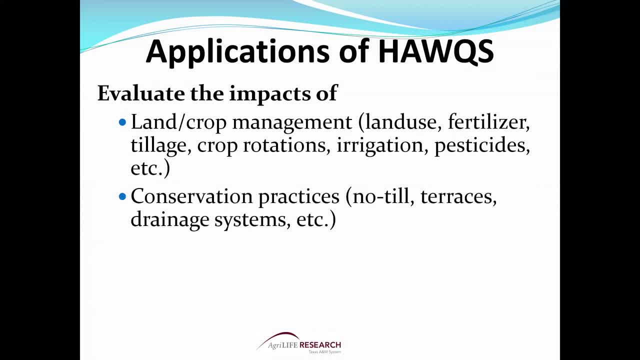 irrigation, crop rotations, conservation practices, pollution control- either it's a point sources or non-points, or load allocation or source allocations. You'll be able to do a lot of them actually, And you can also look at climate change or climate sensitivity or climate resilience. 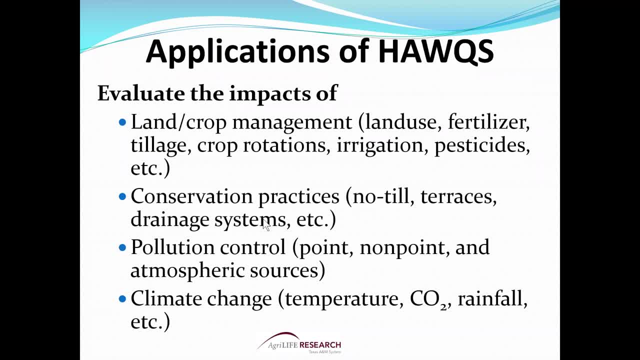 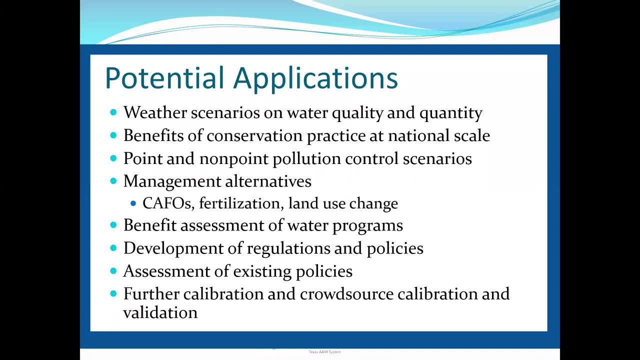 whatever the terminology you are more comfortable with to do any climate scenarios. So these are all. I listed a few other applications that's already been used. The national HOCS for most of them are weather related scenarios or conservation practices, or CAFO operations benefit assessment. 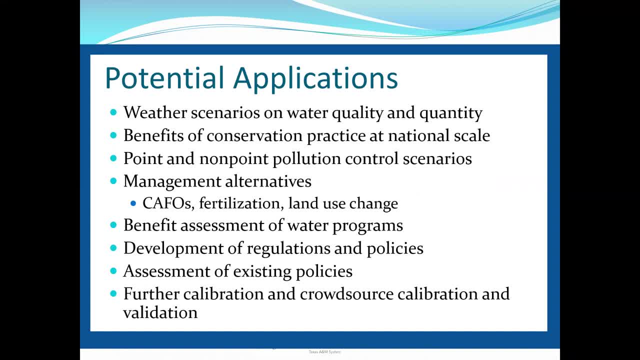 A lot of the time, people who are using a HOCS system are non-hydrologists and water quality specialists used for economic and environmental type of ecologists use the model to look at the impact of water quantity and quality on ecology or environmental environment or economic impact, and so on and so forth. 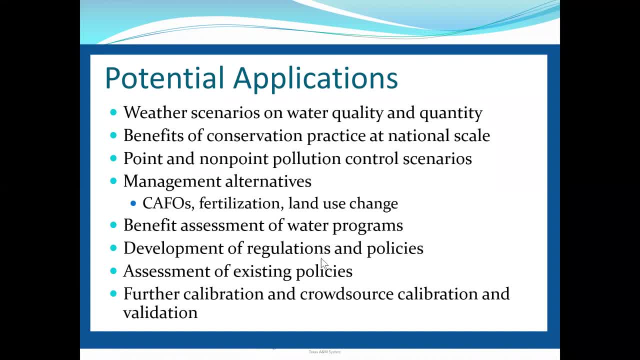 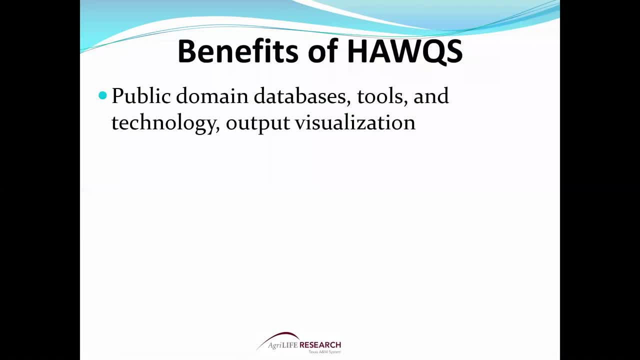 And of course there are lots of regulatory and policy implications- has been assessed with the system also actually. So just to wrap up the HOCS using public domain databases, tools and technology inputting output resolution: no GIS software knowledge required, It's a standard assessment through web architecture. 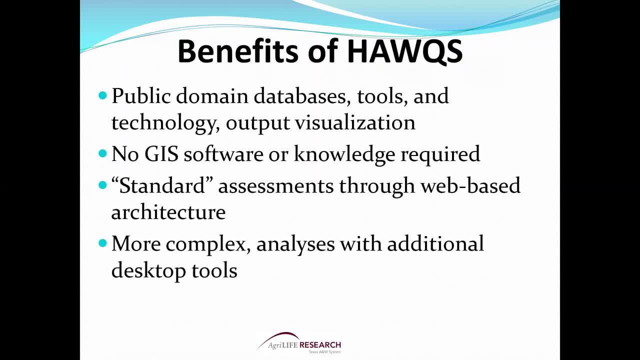 or more complex analysis with additional desktop tools could be done And one of the analysis that was done shown more than 90% reduction in time and effort to put together a modeling system for an assessment. In other words, if you look at a lot of the time. 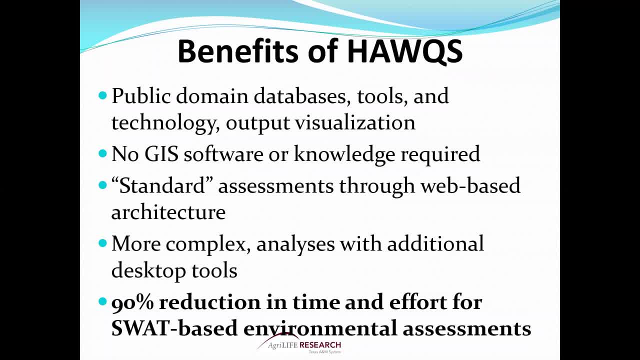 either if it's done for an academic research purpose or for consulting company or anybody else. it takes them anywhere between one to two months just to process all the input and get the inputs right, And then the data set is ready before they can even run. 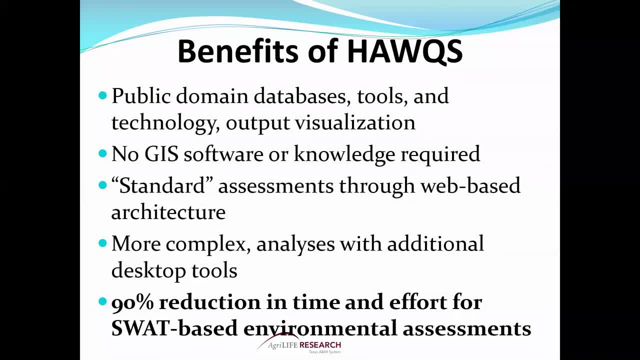 the model, leaving alone calibration, validation and stuff like that. Here you are going to have your data set, That's, with most updated, most detailed available database, including flow calibration for the whole state will be ready And you'll be able to run the model anywhere. 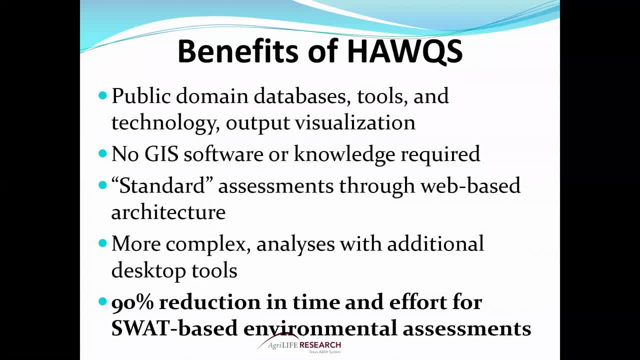 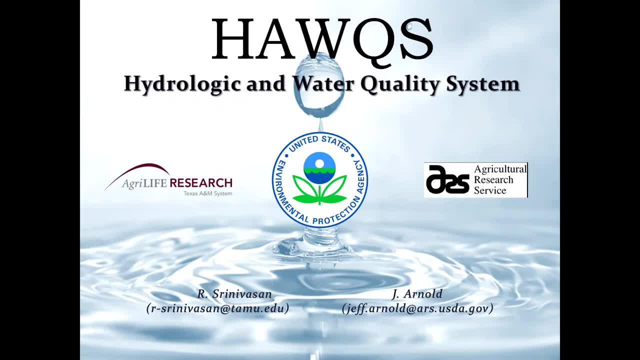 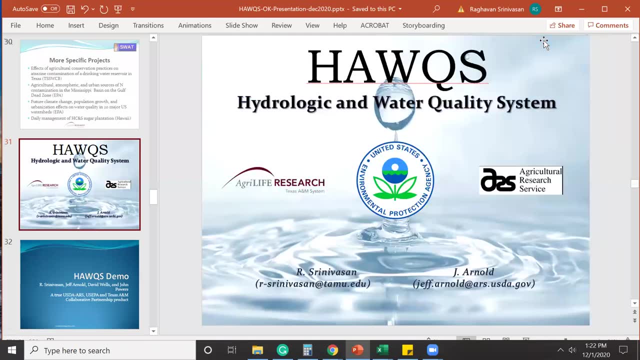 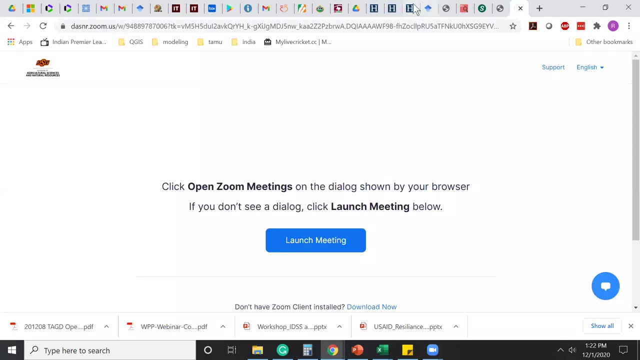 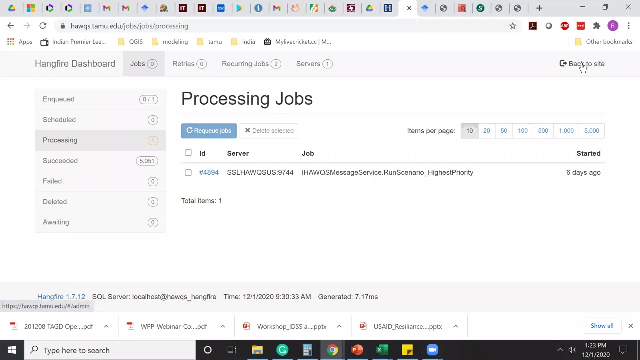 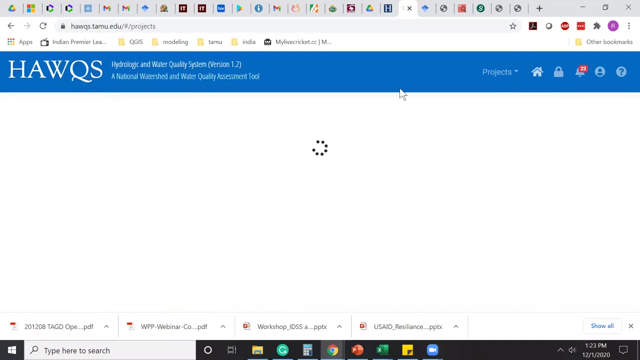 in the state of Oklahoma, within a few minutes actually. With that, let me stop right here and jump into the online system to give you a live demo of the HAWC system. Okay, Sorry about that. So what I'm demonstrating right now as an example, 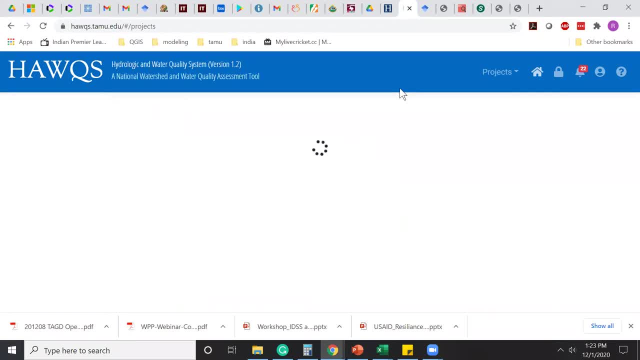 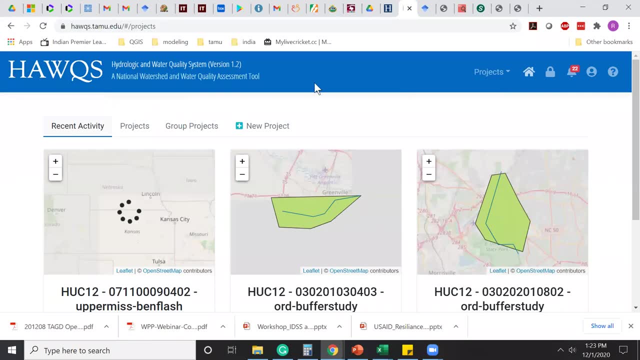 the interface looks very similar to what you're going to see today, But the database, the calibration model and everything will be for Oklahoma HAWC. Okay, So this is obviously a national HAWC. just to give you a preview of what it will be actually. 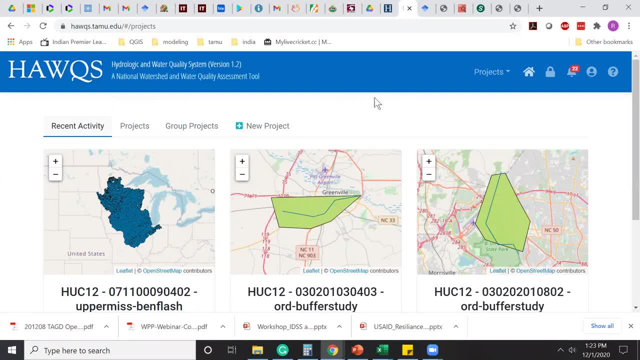 So, if you want to create a new project, this is my desktop here. actually, I'm logged into through Chrome to the server- HAWC server- And let's say I want to create a new project. I simply click here, create a new project. 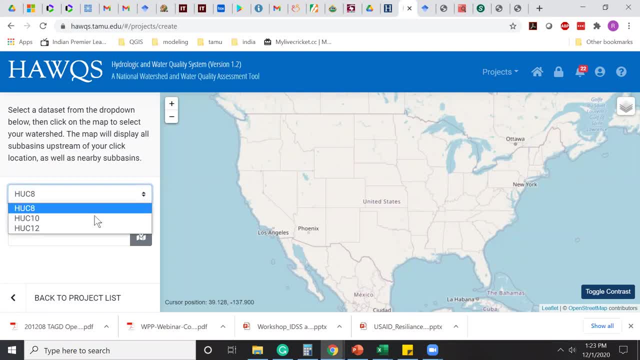 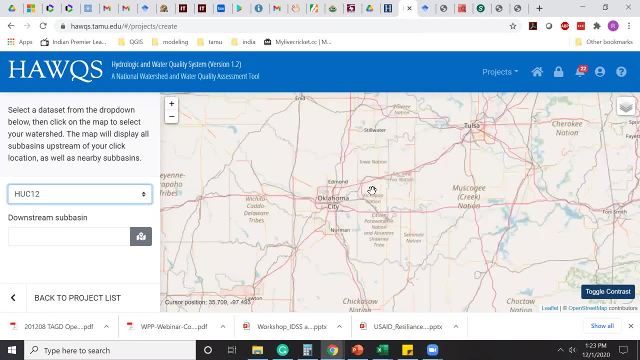 And I'm going to select for Oklahoma HAWC. we are going to have the data available by HAWC 12. And I should be able to zoom in anywhere within the state and be able to select, Let's say, if you want to model this river here. 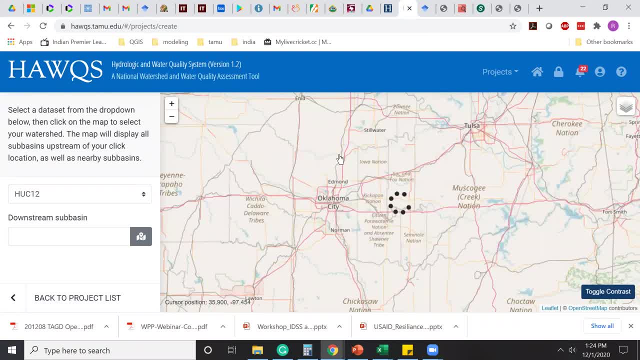 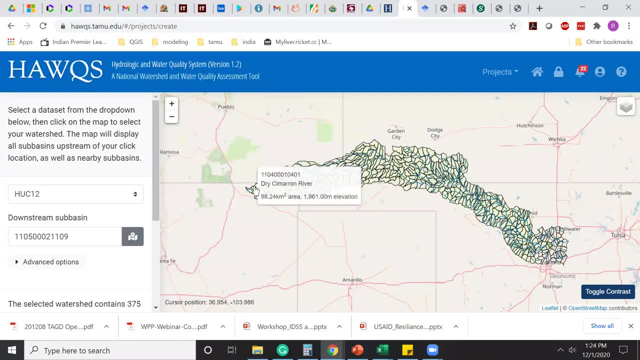 I can simply click on that river. It will automatically draw all the HAWC 12 boundaries upstream of that, actually. But I'm not required or I don't have to, even though now you can see, this goes all the way into Colorado, and so on and so forth. 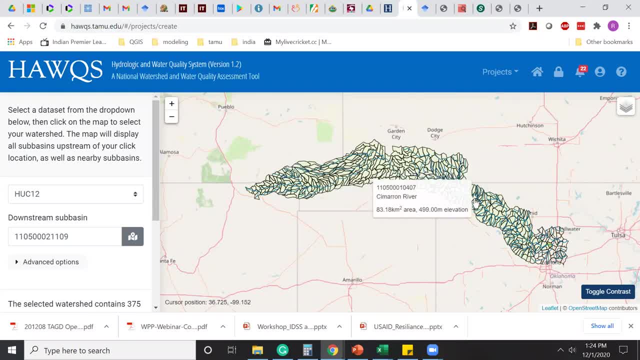 So I don't have to model everything here. Let's say I want to model only from somewhere along the river. Let's say there is a dam and you want to model only from that. I can simply go here and I can go to the advanced option. 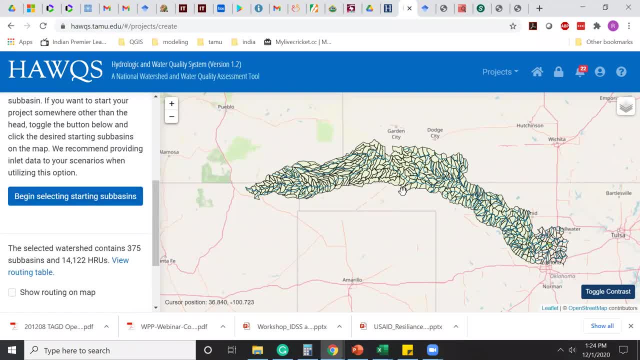 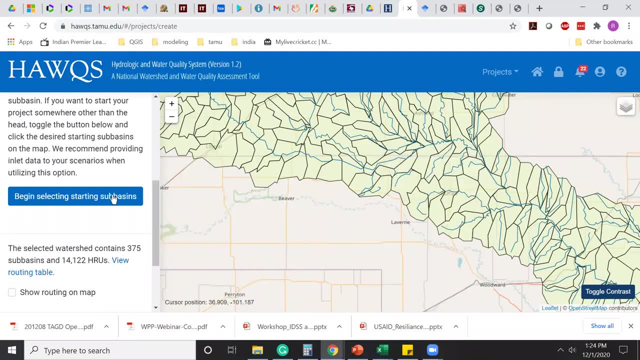 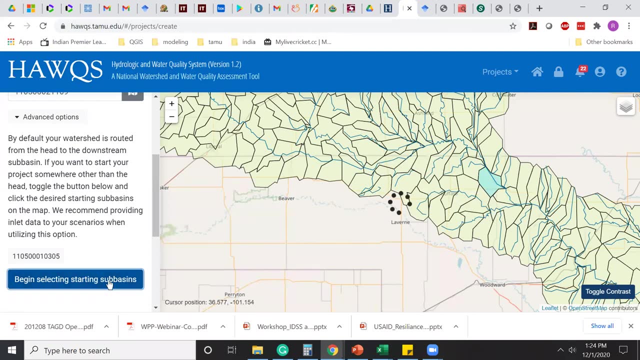 and I can say, okay, I would like to begin my modeling only from the border right here. actually, Let's say, this is your starting point in Oklahoma. Then I can say, simply select that, click on that sub-basin. and I say then, selecting sub-basin. 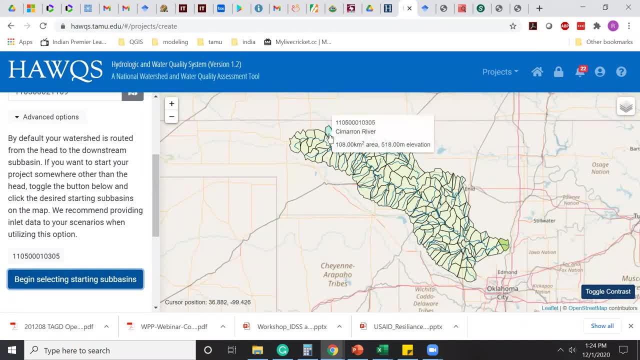 So it will automatically truncate everything upstream of that and that will be a boundary condition to start your river from that, So you can interactively select the area that you want to model. Just because I'm going to do a simple demo, I'm going to choose a smaller river. 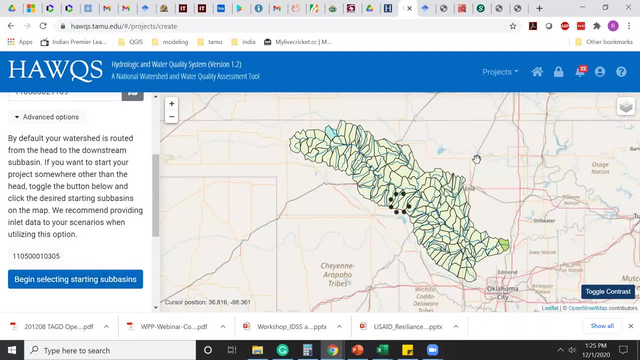 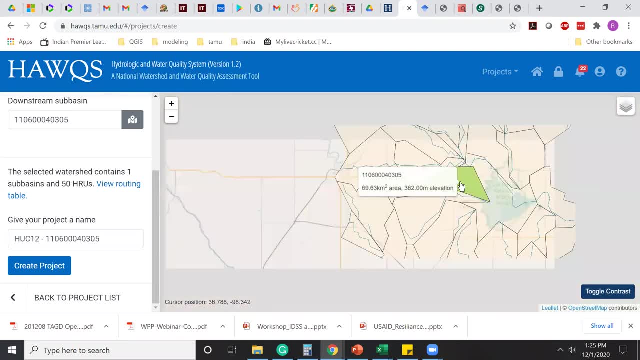 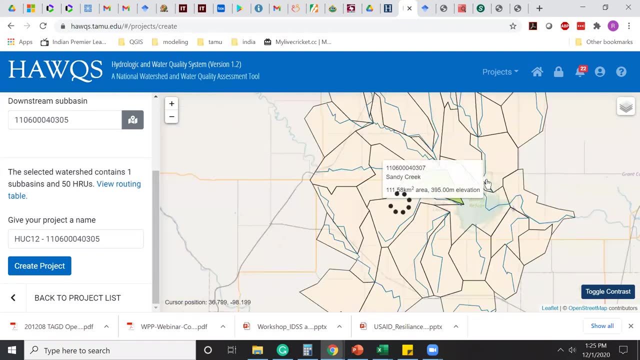 Let's say I'm going to select something like this one. I zoomed in too much. Let's say, I want to model whatever that's flowing into this lake, for example, So it shows you the area that is draining into that lake. 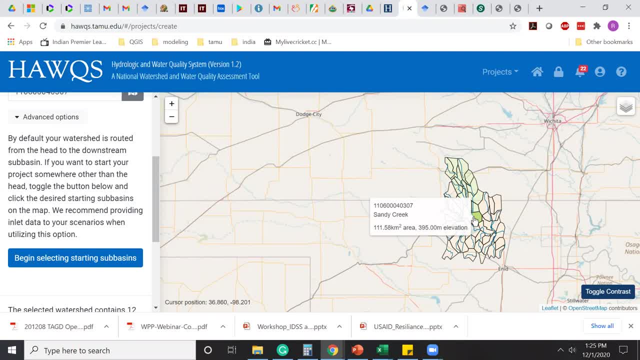 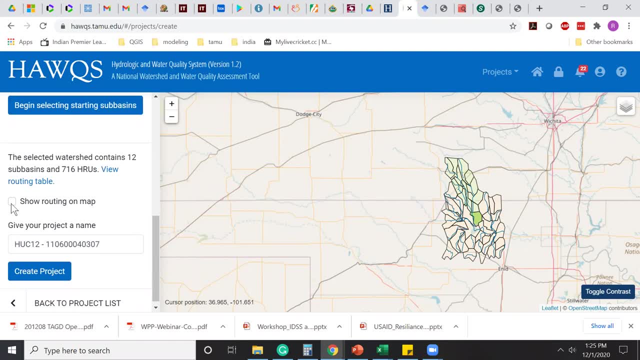 and you can also see the name of the creek and so on and so forth. This is what you want to model. I select that. And if you want to look at the routing, how the water is going to get routed, you can also see that on the screen itself. 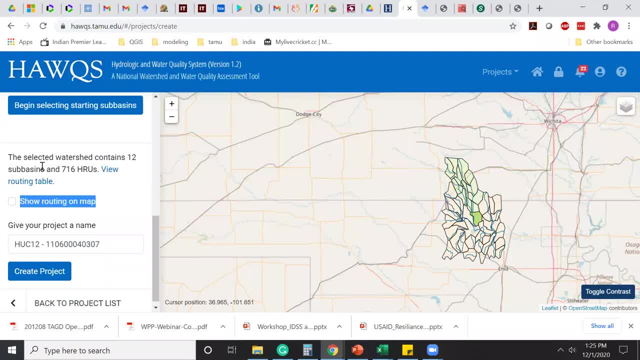 Or if you want to look at the view, you can also look at it. There are 12 sub-watersheds here, 12 HUC-12 boundaries, with 716 hydrological response units, which is nothing but overlay of land use, soils and a slope map. 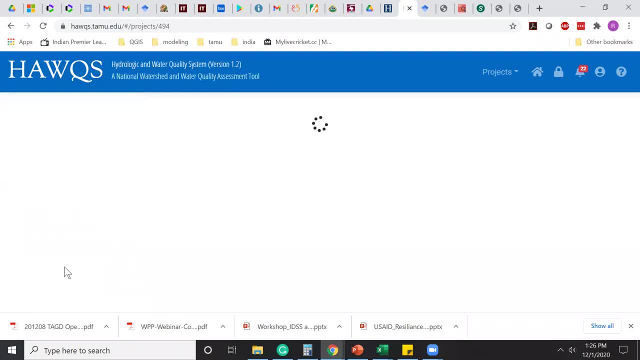 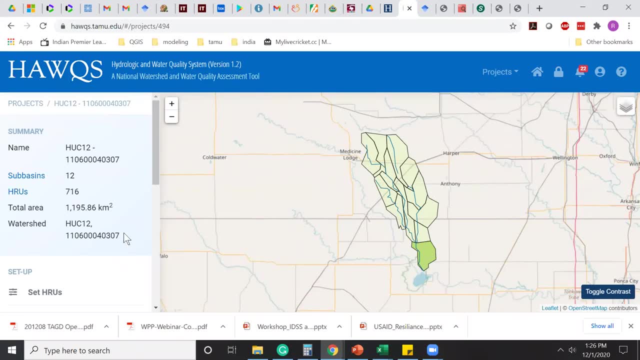 So let's say I want to create this project, I click Create, So now I'm creating a project for just that region that I just selected here actually, So you can interactively select that, and then I'm ready to set up my HRU. 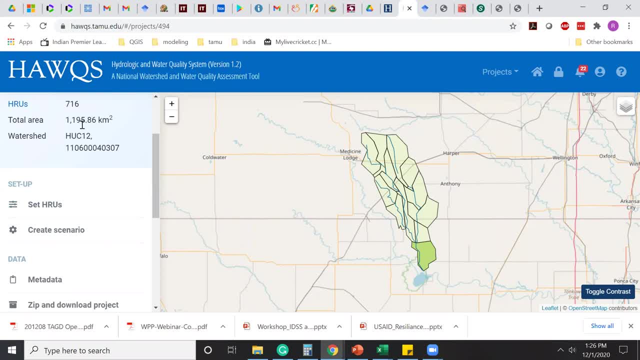 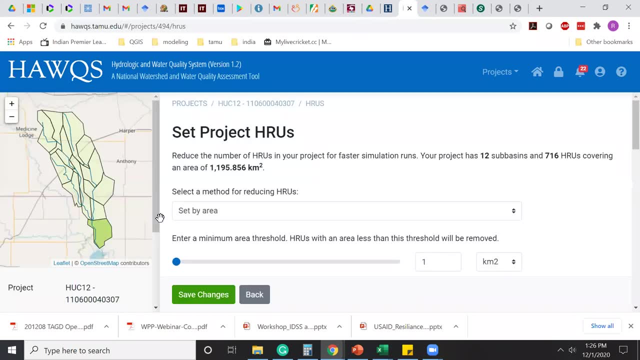 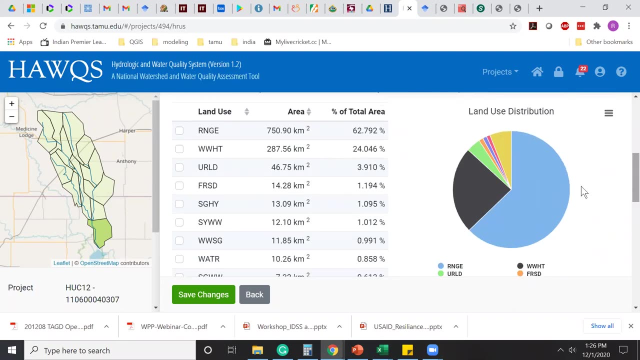 The size of the watershed is about 1,200 square kilometers with 716 hydrological response units. I can look at what are the distributions of land use here actually, So when I click on the HRU, it's going to show me what are the different land uses. 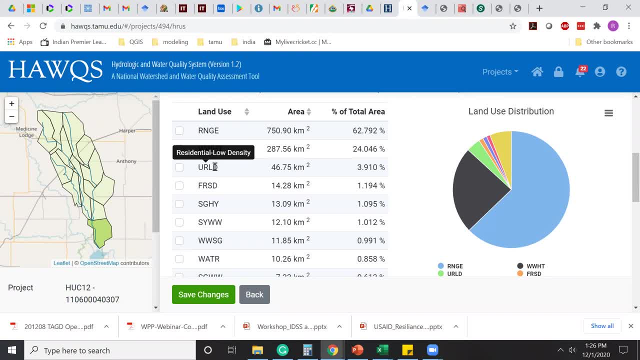 what are some of the dominant ones actually? So you can see about 62% is rangeland and about 24% is winter wheat and then about 4% is urban. If you want to protect any of these land uses, 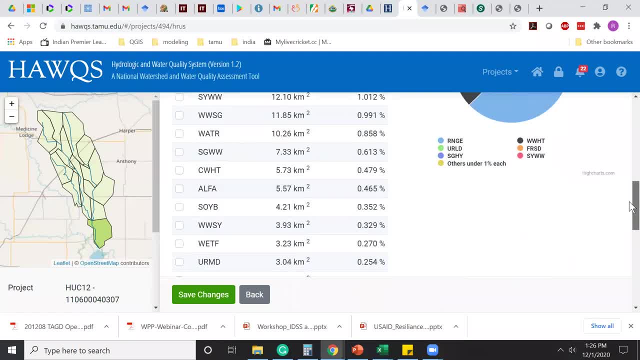 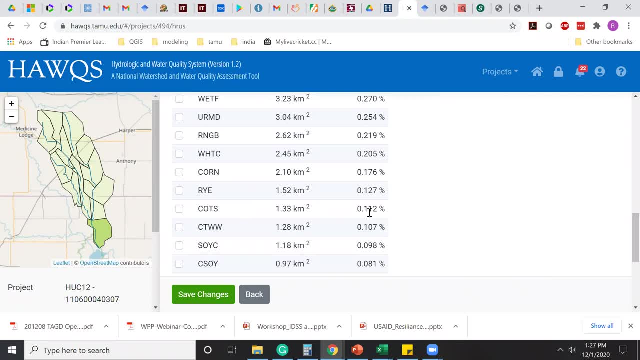 you can protect them. actually, Just because they are very small, they don't have to be like cotton, for example. Cotton is only 0.112% of this watershed And if you felt like cotton is an important crop, you are going to simulate some pesticides. 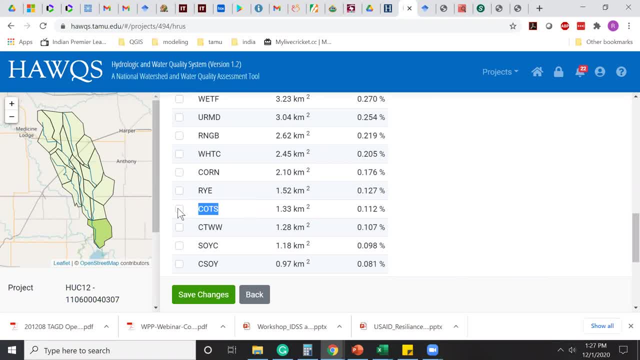 whereby cotton is important. You can just select this. That means it will not be subject to any elimination. So anything that you check here, that means don't remove that land use or don't remove that HRU, You don't have to remove anything actually. 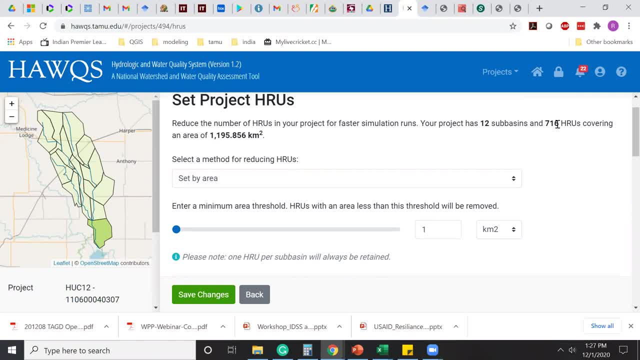 I can set up this to 0,. thereby I can model all the 716 HRUs. But sometimes, because when you overlay the GIS layers, you may have some sliver polygons, like one or two pixels, that you may say you don't want to model, 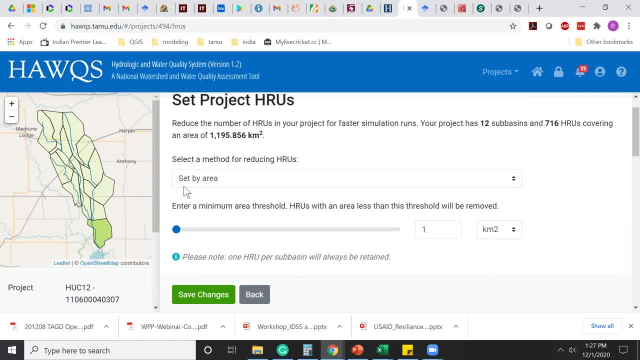 that one to two pixels actually. So you can set up threshold, like I said, by area or you can target number of HRUs You set by area. You can say, okay, I want to consider at least a minimum of one square kilometer. 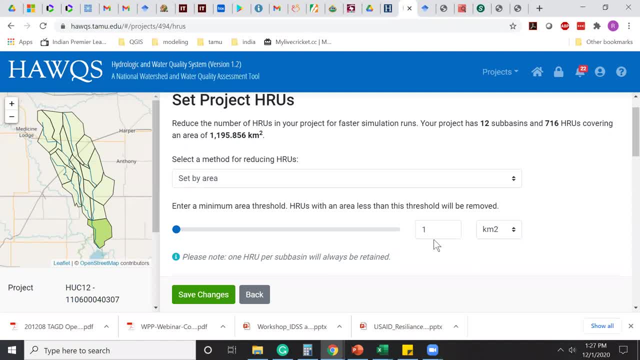 That means out of the 1,200 square kilometer. if your HRU is not even one square kilometer, it will remove that HRU and aggregate with the rest of the watershed. We are still modeling the same 1,200 square kilometer watershed. 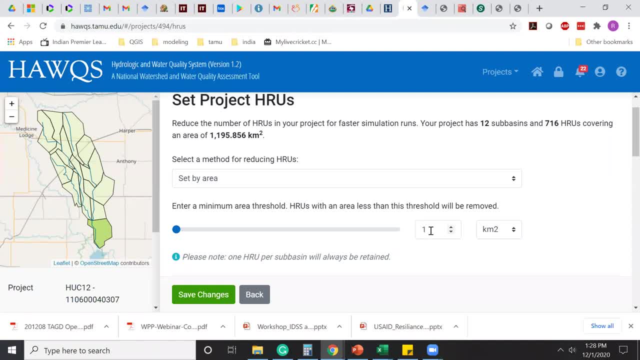 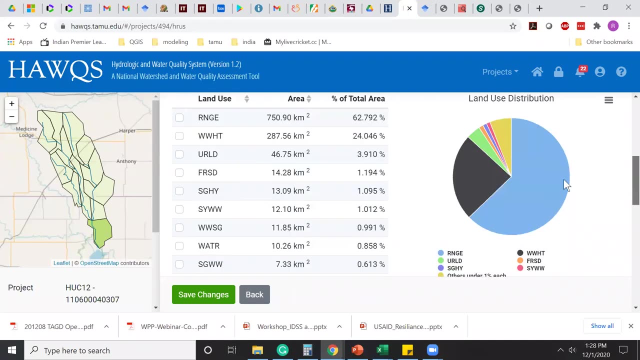 but it will remove the smallest polygons or smallest area that is less than one square kilometer and aggregate that to the rest of the HRUs so that by proportion, when I say proportion, it's proportionate. based on what is it actually? what is the weighting factor? 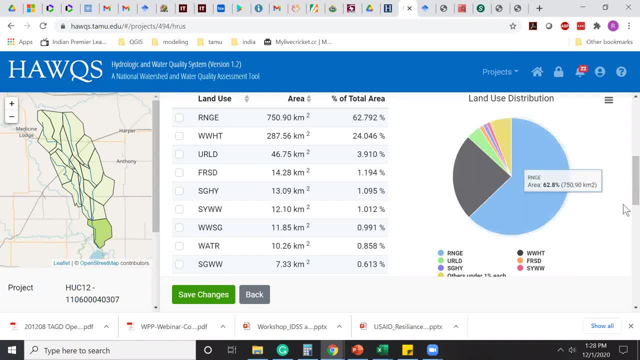 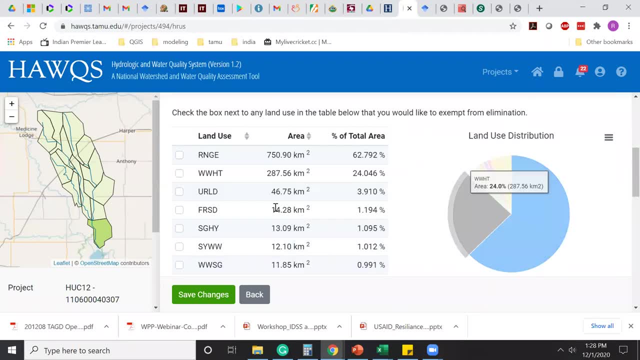 the weighting factor. The weighting factor is the percentage of the area that occupies the land use in that subbasin. So, again, this is only optional. If you don't want to use this step, you can directly use all the 716 HRUs. 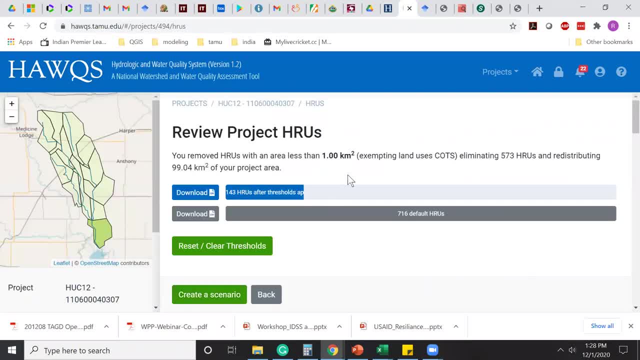 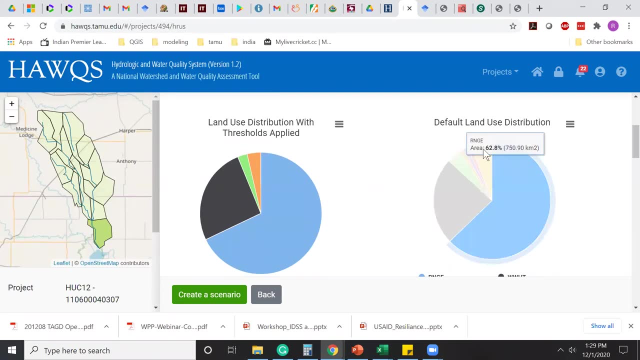 So let's say I save the changes, So it's done So now. it eliminated about 573 of them at less than one square kilometer and it did protect the cotton landscape, thereby. the new: this is the original distribution and this is the new after you apply the threshold. 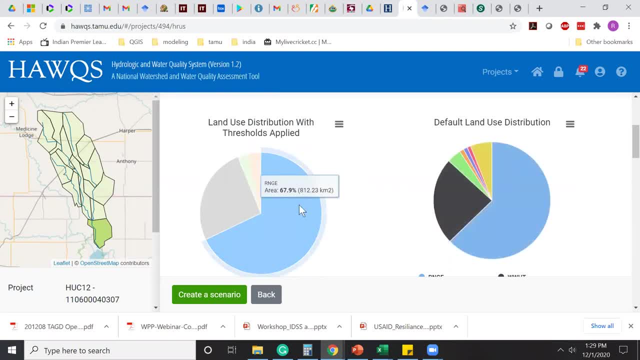 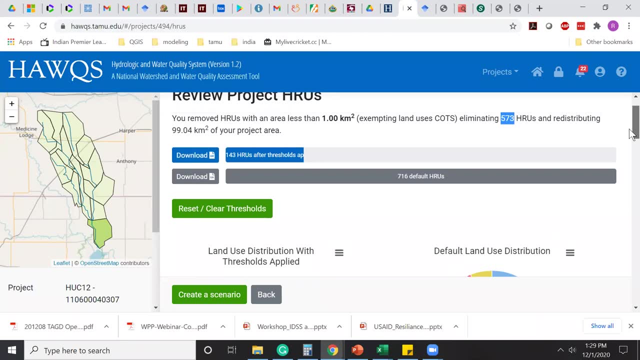 So, if you look at it, 62.8 was range, Now that's become 67.9.. There are a few percentage points has increased because of the lot of small, small, tiny polygons due to the overlay of land use and soils and slope maps. 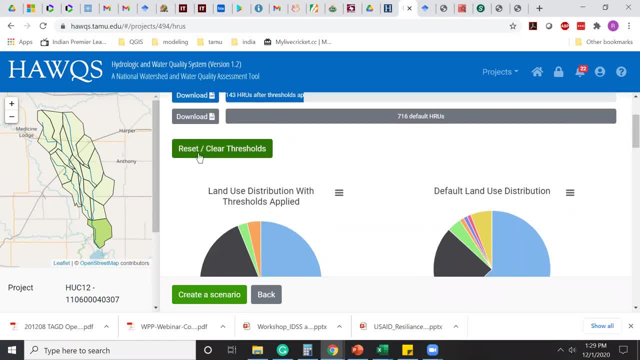 Okay, Again, if you don't approve of this, you can reset the threshold, go back and redo this analysis if you want. This is just a demo, So I'm going to go ahead and accept this and say: create my scenario. 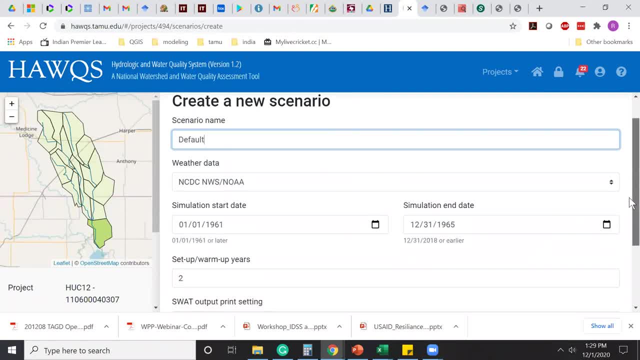 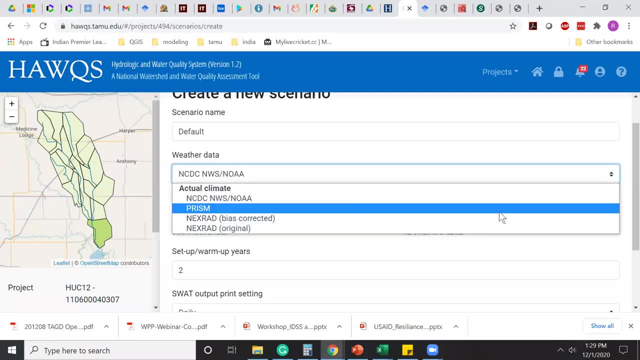 So here is a scenario that's going to develop. You can name anything you want and then you can choose what weather data that you want to choose to run your model. Okay, Let's say I want to run Prism, for example. Okay, 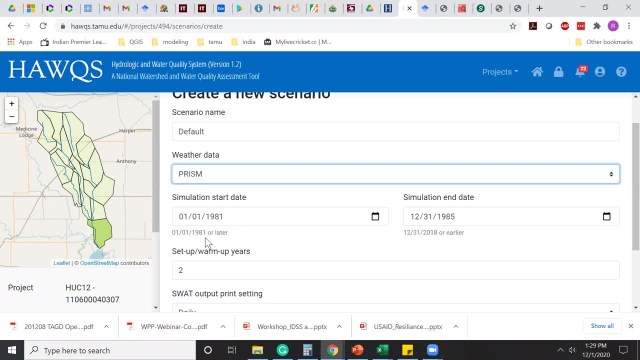 And the Prism data set is from 1981 until 2018.. We'll have until 2019 shortly. Let's say I want to run, that You don't have to run all the 38 years. You could say I want to run from 2008 to 2018,. 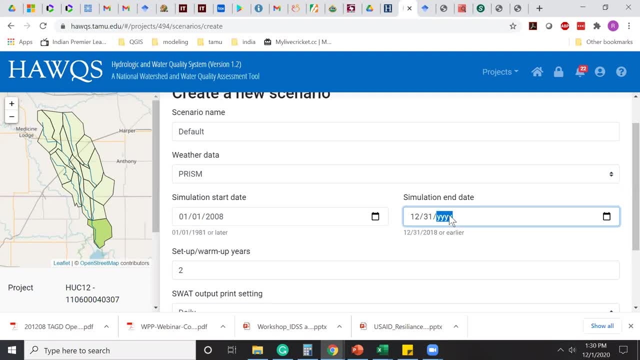 for example, the last seven years, Sorry, Okay, So you can choose only, or you can just click on here and you can do a calendar model. So actually I'm just typing it directly And you can set up your warmup period. 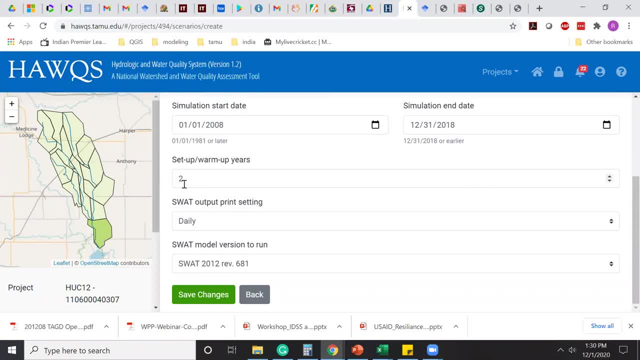 however many years you want to set model setup period. That means the SWOT model will not provide your output for 2008 and 2009.. And it'll give you output only from 2010 to 2018, depending on how many years you are considering. 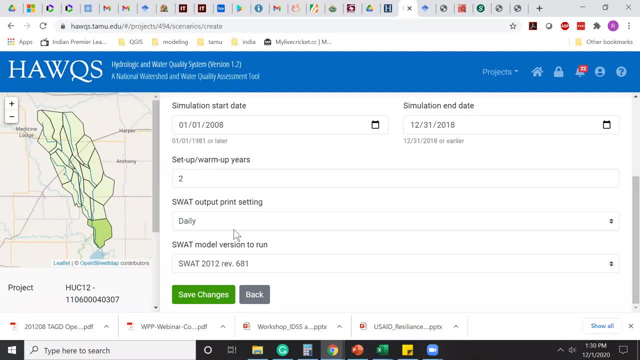 as a warmup period or setup period, And it's going to give you a daily output or you can ask for monthly or annual output, And you can also choose which version of the SWOT model you want to run. So one of the nice thing about the HAWC system is: 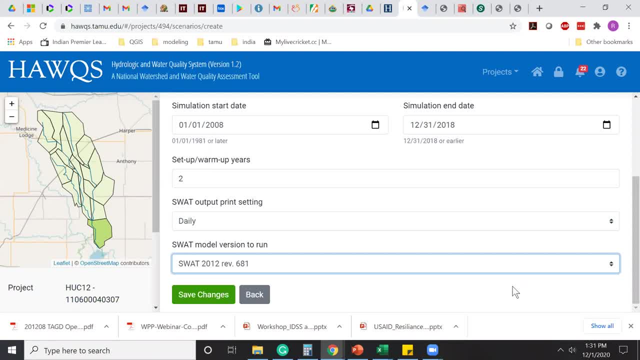 the entire system, the entire modeling is online archived, So you don't have to worry about saving your project or anything like that. Let's say, if people move from job to job and if you are in a company consulting company, 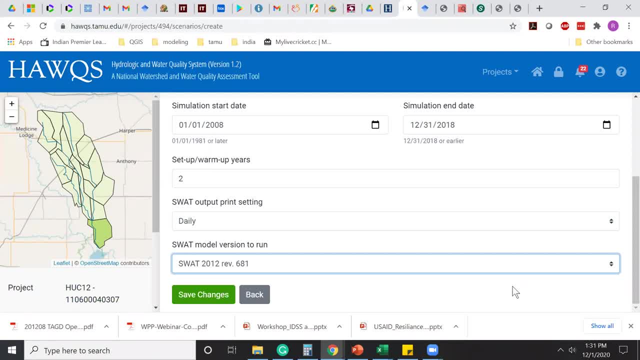 and somebody has moved, the project still stays on the system, So thereby you could easily go back and be able to recline that project and able to do an additional analysis. Let's say, five years from now you want to do additional analysis. 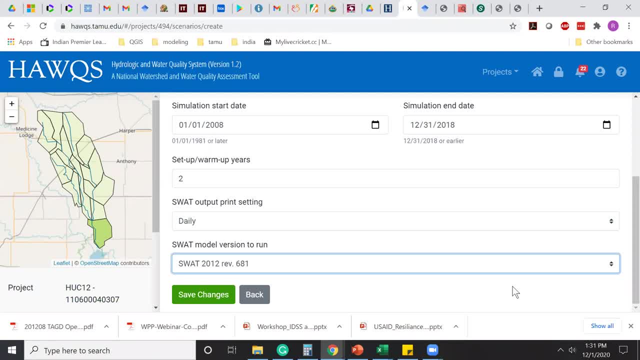 another project, another scenario. you don't have to build from scratch. You can go back and dust off the old project that you created and able to even run the old version of the SWOT model if you want to, and then able to run scenarios. 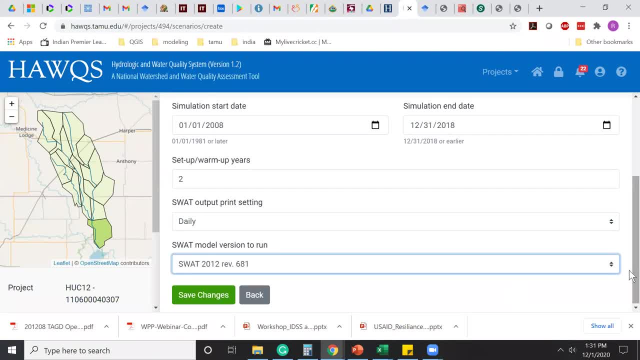 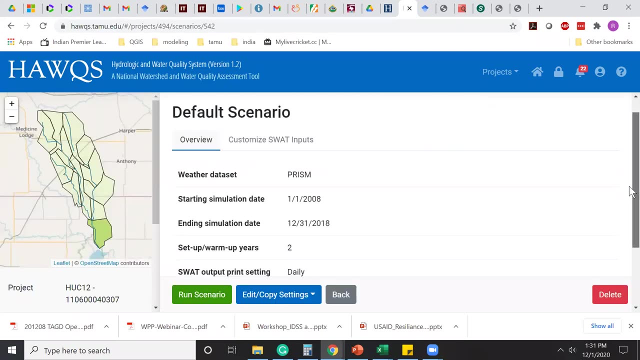 So that's. another nice thing about this is it's all completely archived and reproducible results, which is one of the requirement for any water quality and watershed project. So once you set up your baseline- I mean the model inputs for the time period you want to run, 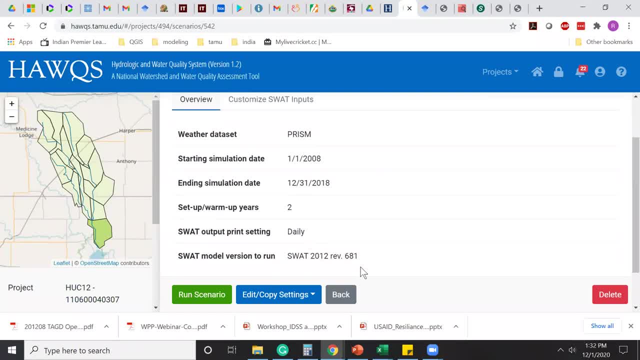 and what weather data you want to choose, how many warmup period and daily output and what version of the model. That's all it requires to set up the model actually. Now I can say run my scenario. Before I showing the running scenario. 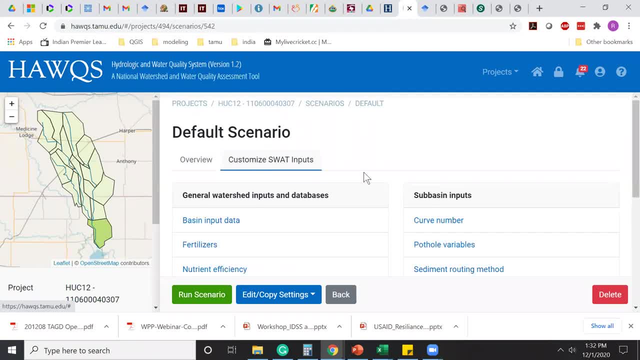 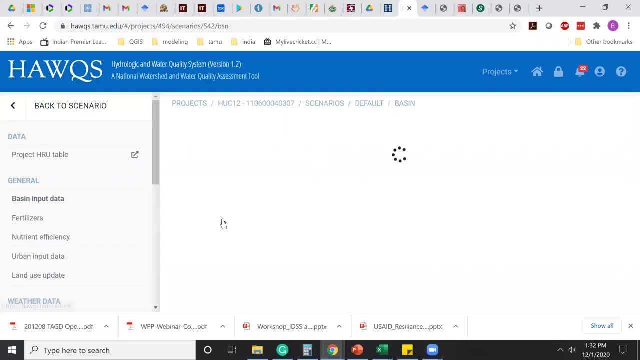 I also want to show few inputs that you can customize. For example, you can customize the basin level input data set. You can go in here and you said, oh okay, I want to. I don't want to use Spendman method actually. 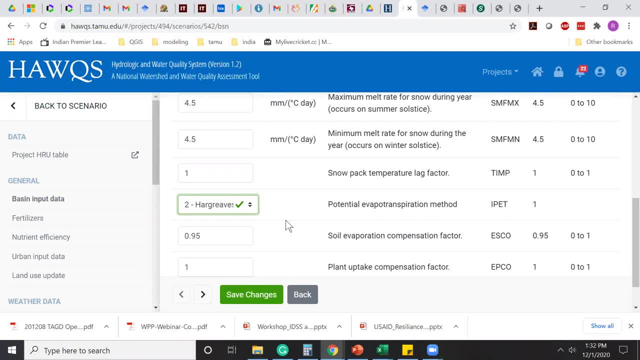 and I really would like to use Hargrave method, for example. You can change it, You can change your evaporation factor. if that's an important to you, Then whatever changes you make, you click save changes. that change is made. 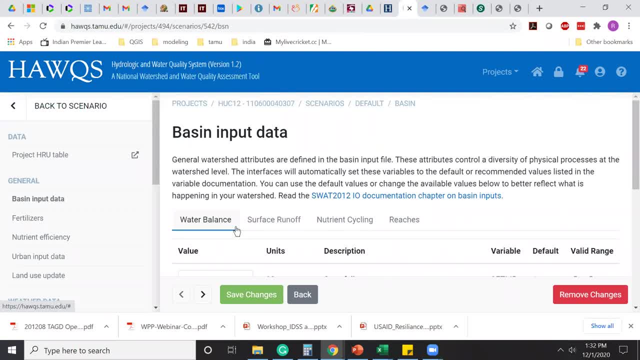 One of the nice thing about the Hawks is it keeps track of every change you make as a metadata. So when you export your metadata you will see how the model was built and how one of the changes were made, so that it becomes a history of all the information that you made. 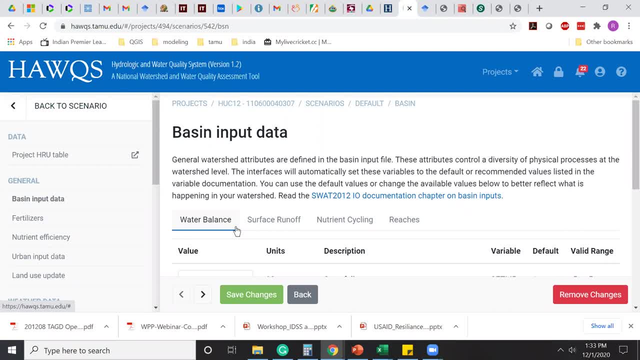 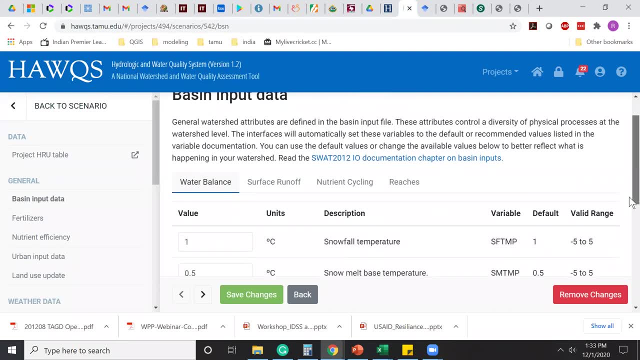 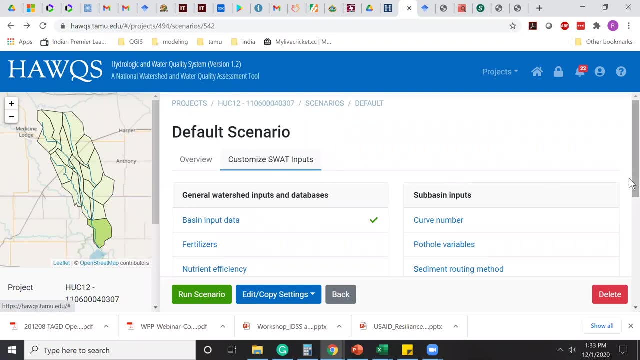 So that again, going from one user to which are going to share models, everybody knows what was done to that inputs to generate or to create that model. So you can do the same thing in other inputs here, or I can go back And if I want to change my current number in the model, 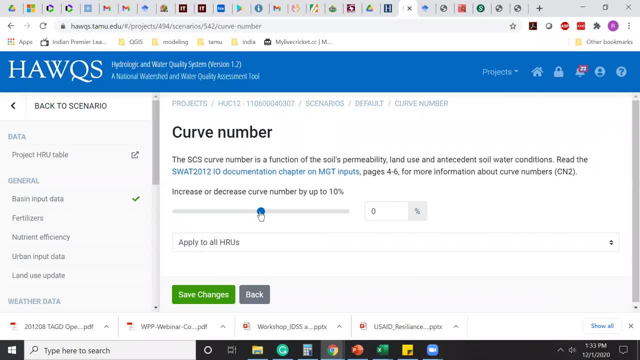 I can simply go to current number And I say, okay, I want to increase the current number by 2%. You can do that. You can apply to all HRUs or specific HRU. So when I say specific HRU, you can select okay. 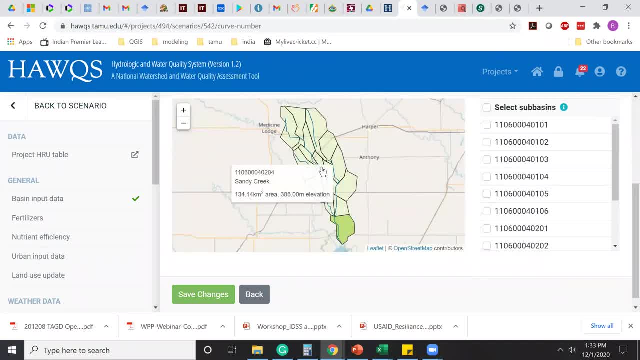 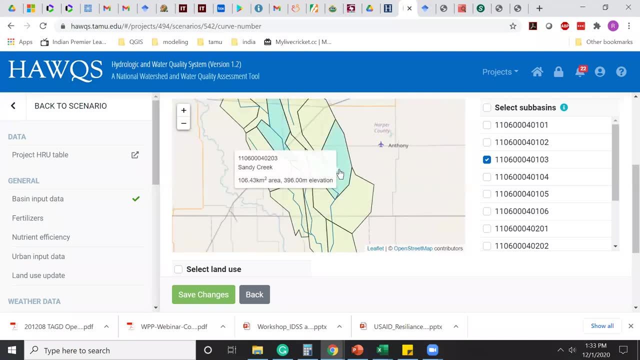 where exactly you want to make the changes, which sub-basin You want to apply to that sub-basin? only that sub-basin will be selected here, Or you could select multiple sub-basin, for example: Okay, And then within that. 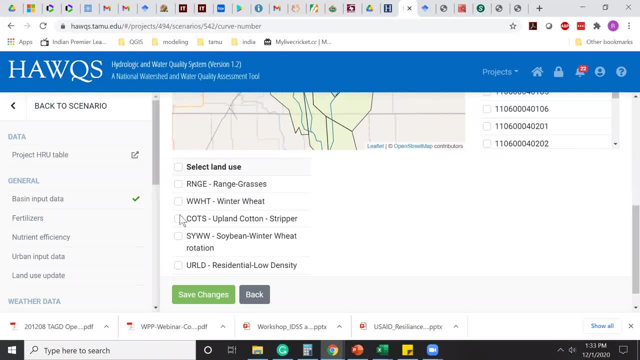 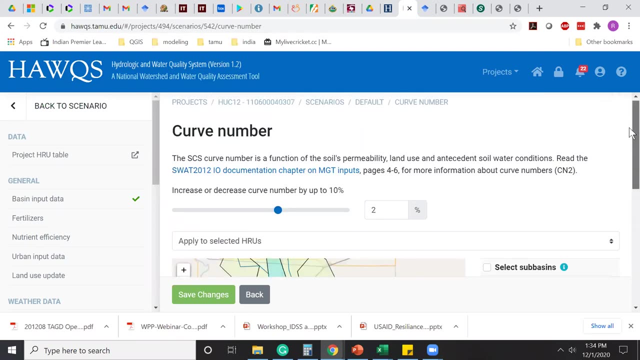 you can also select what land use you want to apply, to What soil, what slope, So you can go and change input on a specific hydrological response unit or specific landscape, or to the entire watershed, depending on your input choice that you want to make changes. 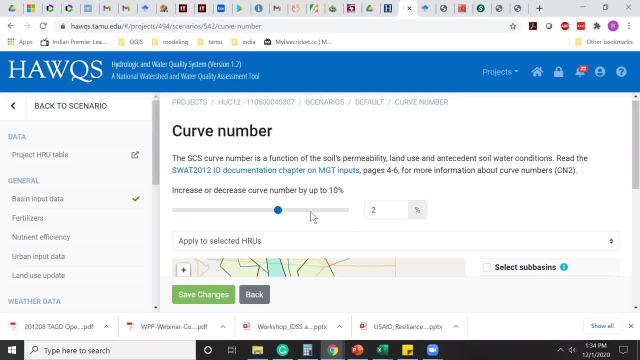 I'm just trying to show you this as an example here. I'm not going to make the changes right now, but I'm trying to show you how you can edit and customize your input to the level of detail that you are interested in actually. 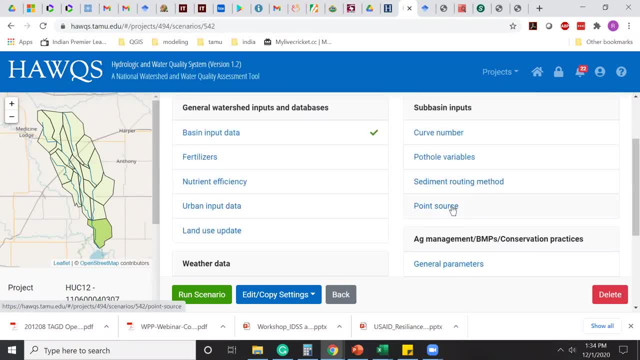 Same way, we have sediment routing models, sediment routing methods, point sources. You can update your point source, your own point source. You can also do land use update, meaning change the land use over a period of time. You could start with certain land use in 1980s. 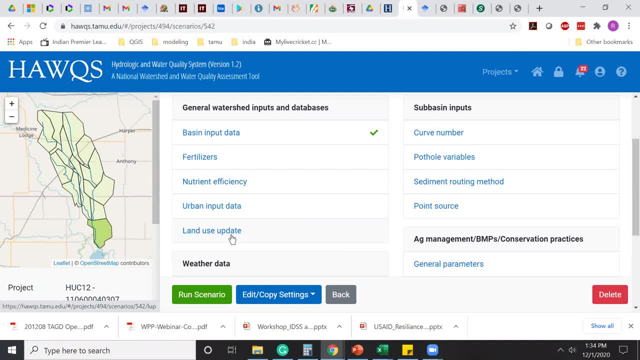 and you can update the change in land use in 90s and 2000.. So you can have a dynamic simulation as the land use changed from over a period of time actually, And you can change your urban data, fertilizer data and so on. 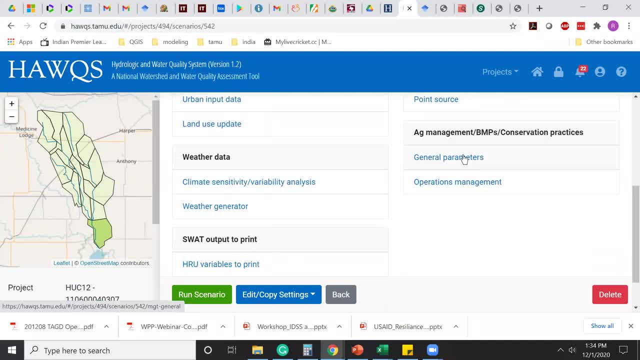 You can also change any of the ag operation, like tillage, fertilizer, pesticides and so on and so forth. You'll do it through here. actually, In the interest of the time, I'm not going to go through that right now, but later we are planning on having. 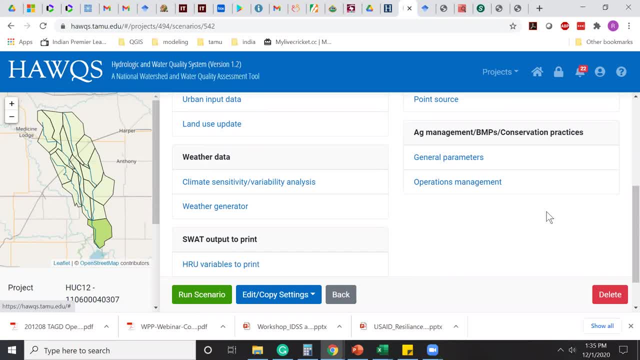 a full blown workshop of using Oklahoma hawks. So at that time we'll be able to run various scenarios, building a model and so on actually. So I think we are expecting some time in March, April, springtime- we will have a follow up full blown workshop. 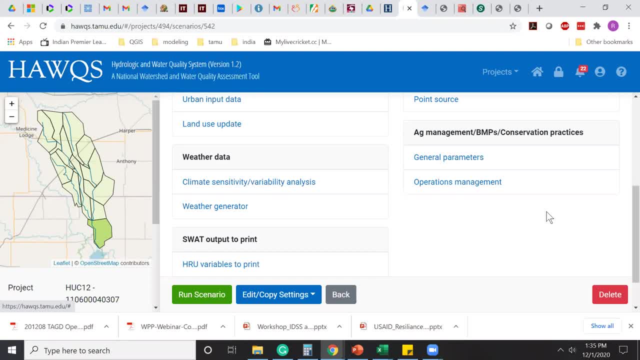 a day long or a half a day to three quarter day long workshop to go through this inputs and go through the various scenario, building and so on and so forth. Okay, Let's say you are ready to run the model, So you can say: run. 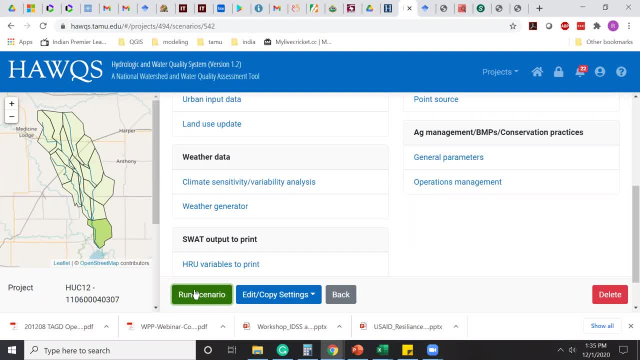 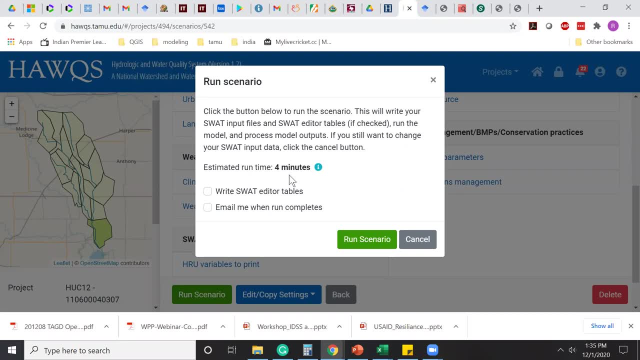 My mouse is very sensitive. Give me one second, Okay. So so it gives you enough time, is about it's going to take about four minutes. I don't think it will take that much time. So you can see this. next option is edit tables. right? 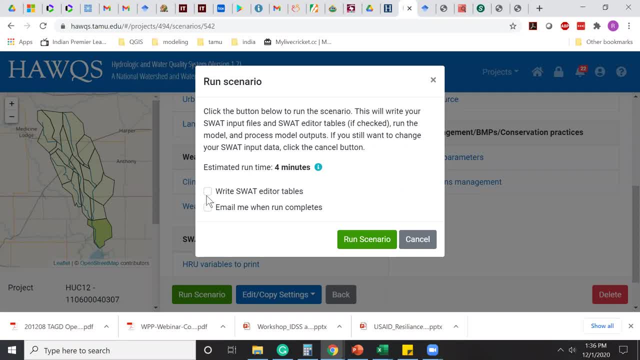 If you choose this option, you can download the data and run offline. That's the only reason you want to choose this option. If you're not going to do that, you don't need that, And also I told you that you can click here. 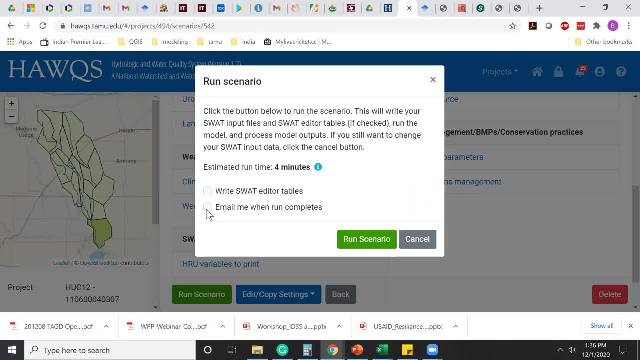 to email you every step of the process so that you don't have to wait on the screen for that process to complete. Let's say you are going to do something that's going to take 20 minutes. You don't have to wait on the screen- 20 minutes actually. 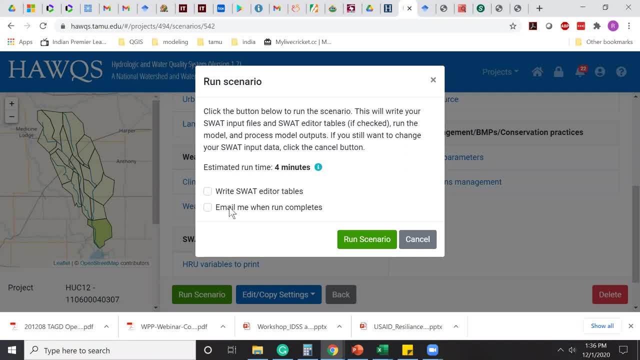 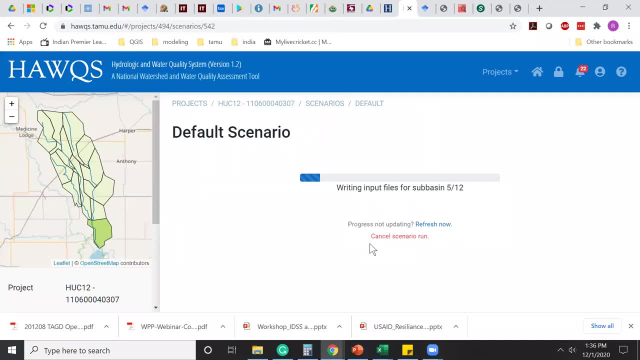 Just submit the job, walk away. It'll send you an email when it is done. Since this is a small amount of watershed, I'm going to go ahead and accept it. And you can see this is starting to write the inputs and it'll start to run the model very quickly. 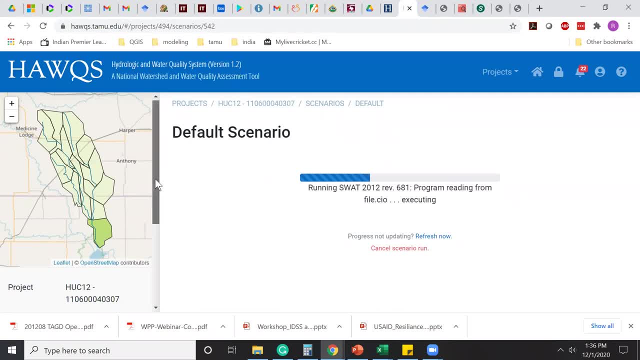 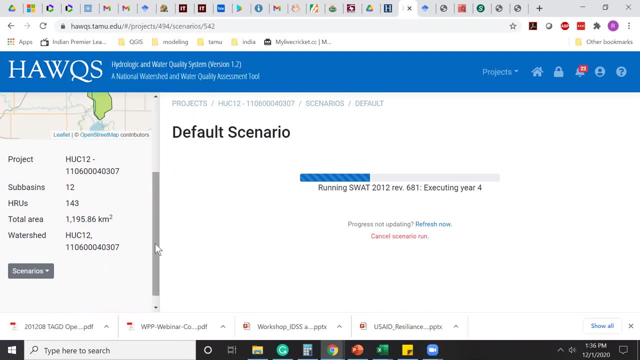 following that actually. So it's right now executing the model. Now there was some question. Maybe I can try to answer that question while that's running. Okay, Are the initial default inputs related to the geography selected for the analysis? Absolutely yes. 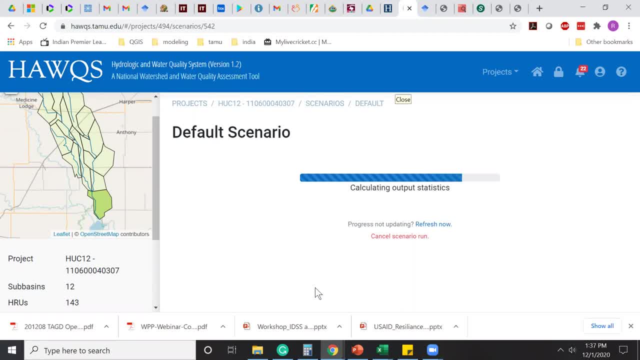 Because these are all geospatial data set, like your land use map, your soils map and your weather input. Everything is geospatial, Everything is geographically specific data set, So all the data will be based on that geography, wherever the watershed that you're simulating. 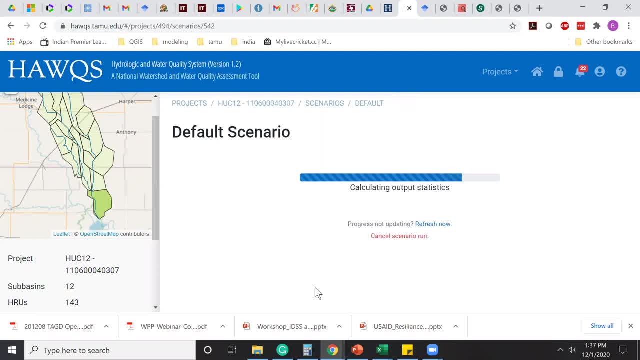 In addition to that, since we are calibrating based on 42 gauges, what you are getting- the initial parameter- is already a calibrated model for that level of calibration. It may not be calibrated on every edge of the form or every small watershed, every HUC-12,. 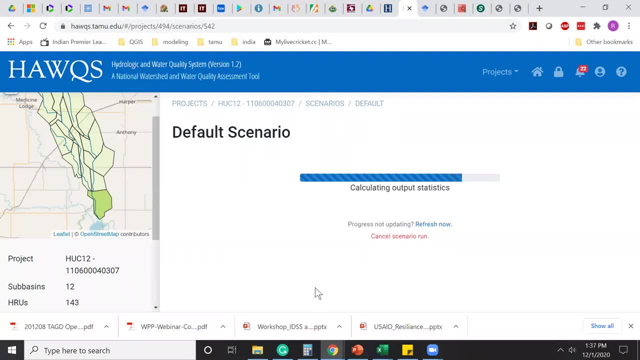 but based on the available USGS gauge. we are attempting to calibrate for a long time period And that will be the basis for the input in the Hawkes Oklahoma version. When you set up your model, you are getting a calibrated model or hydrology. 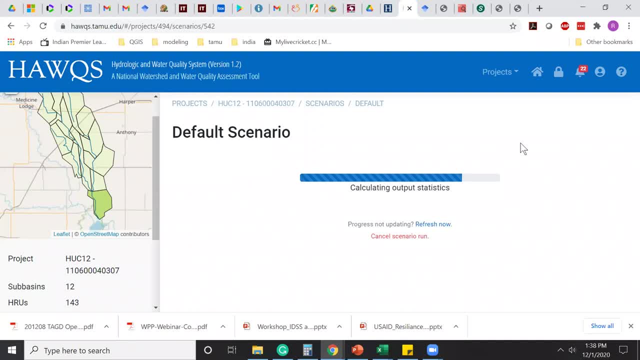 Few more minutes. It's calculating all the statistics and so on and so forth. It will be useful to do the analysis. If there are other questions in the meantime, you can throw in the chat box. I'll be happy to share with you actually. 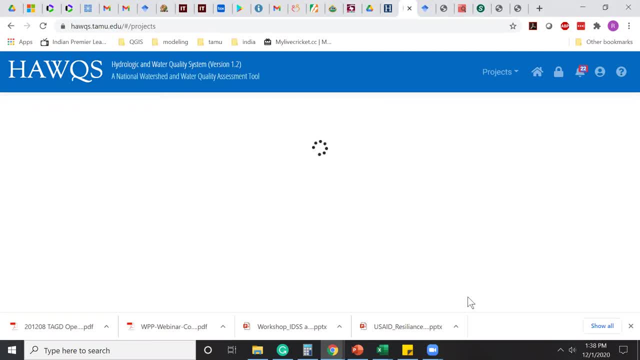 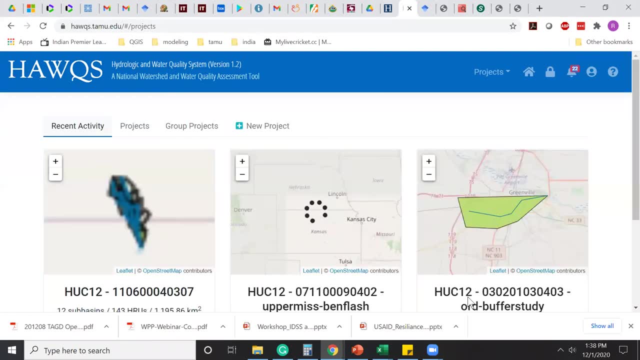 How about coefficients? Coefficients is part of the calibration parameter, right? So when you calibrate, like evaporation coefficient, if it is calibrated for hydrology, you will get that calibrated. So that's the model output. actually Can soil health practices, such as cover crops. 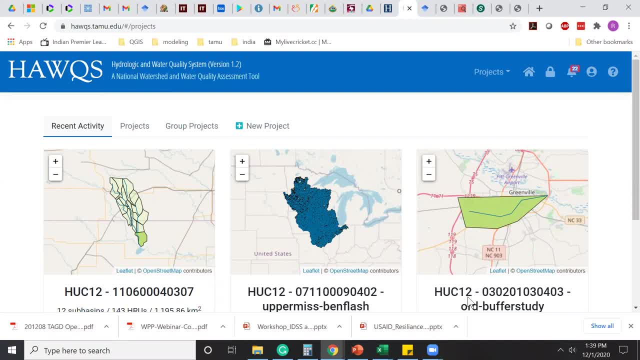 no-till can model. Absolutely yes. So that's what I was showing you about the ag practices. So under the ag practices you'll be able to run them and then you're able to compare the two different scenarios, the current and no-till scenario, for example. 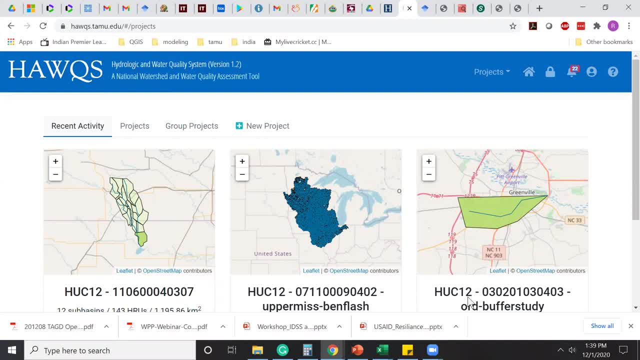 and look at the impact on soil nutrients or soil organic carbon, or look at the sedimentation process and so on and so forth. Are there online training for this program For the HAWCs? we do have a help section. actually, When you go to this help section, 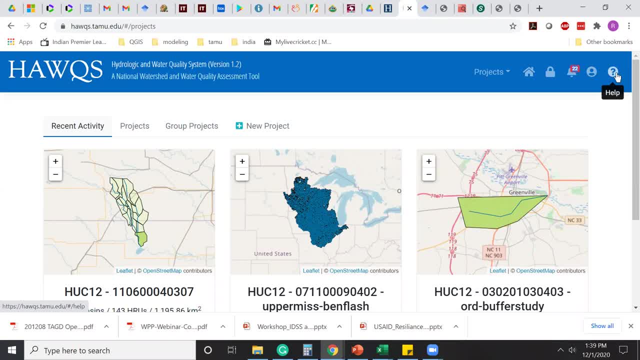 you do have some training videos as well as PowerPoint and documentation and so on and so forth. It's extremely well detailed documentation that's available there, actually, And as we complete the Oklahoma HAWCs, we will have similar kind of thing detailing about how the data was processed. 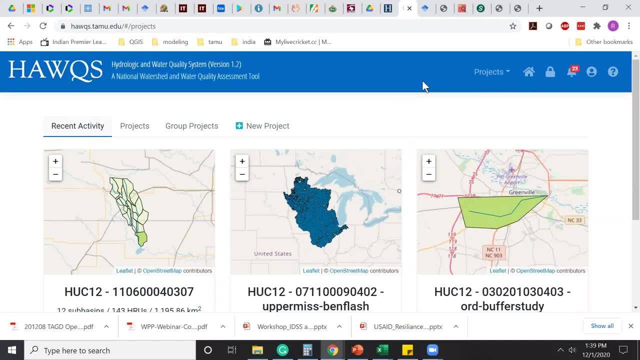 and how the calibration was conducted and what are the calibration statistics. All those things will be provided as part of the modeling system so that you will be able to evaluate whether that's good enough or you need to even calibrate further, or you ought to use some assumptions. 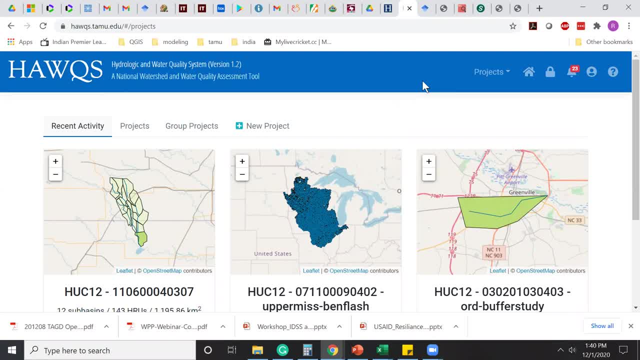 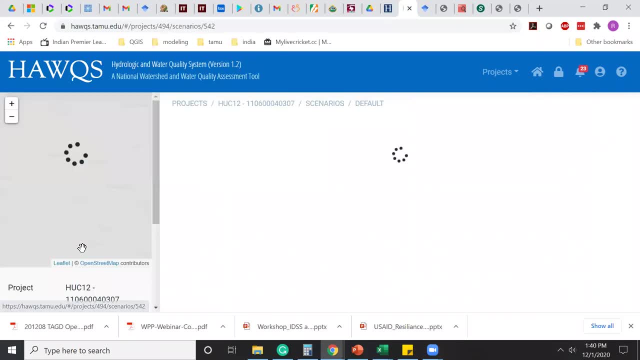 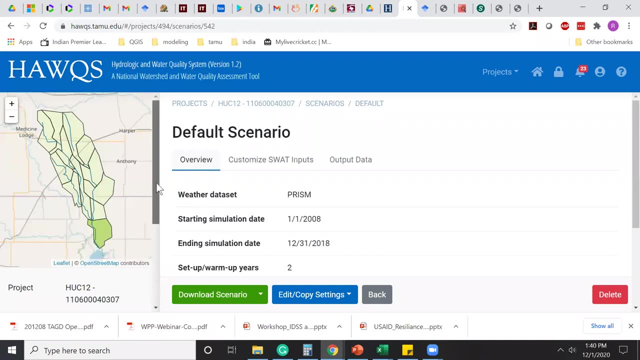 different assumptions. You'll be able to choose how you want to use the system. Okay, I think it's finished. Oh, it's still running. Let's see whether. Oh, it's finished. yeah, Okay, Okay, so the model is run for the 11 or 12 years. 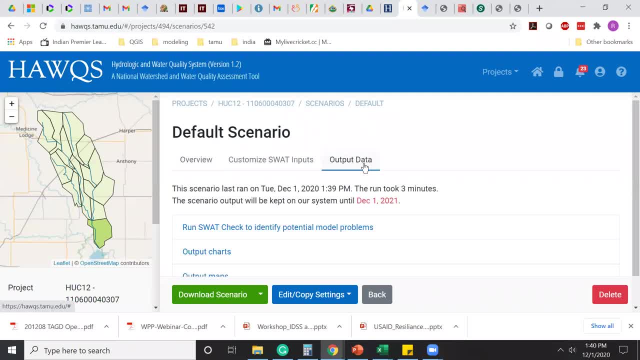 Now we are ready to analyze the output. So when I click on the output I can run SWAT check. Those of you familiar with SWAT model, they may be familiar about the SWAT check program, which is nothing but a 30,000-foot overview. 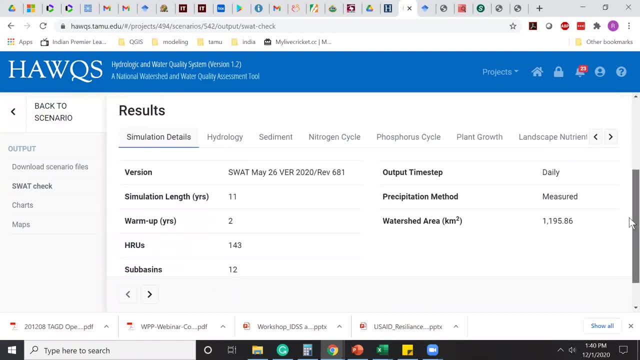 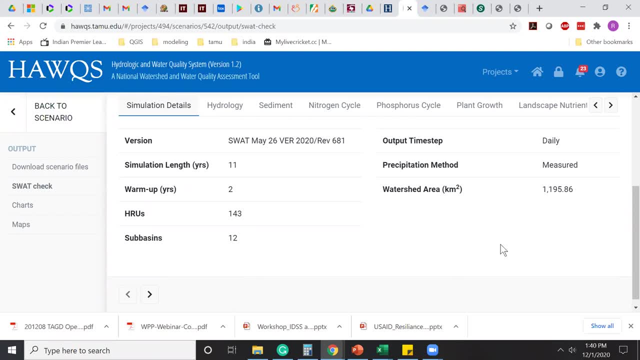 of your watershed, actually watershed analysis. So we ran the model for 11 years with a two-year warm-up period for 143 HRUs with 12 sub-basins, About 1,200 square kilometer watershed. Let's look at the hydrology. 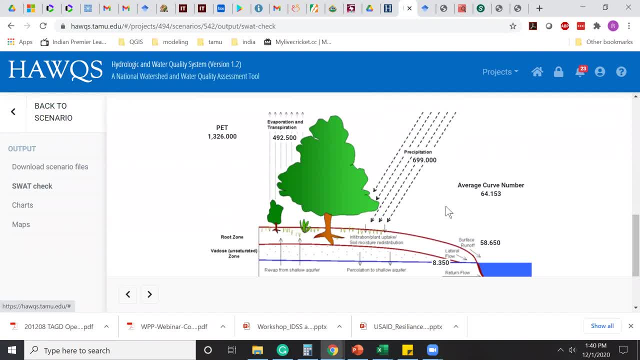 So here is the hydrology. The average rainfall in that region is about 700 millimeter for that period of 11 years that we ran the model, And the average evapotranspiration is about 492 millimeter And the average current number used. 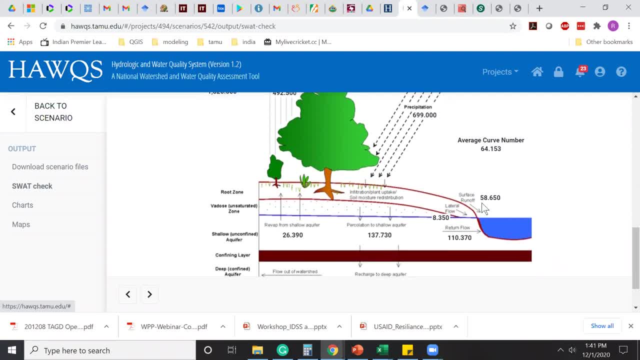 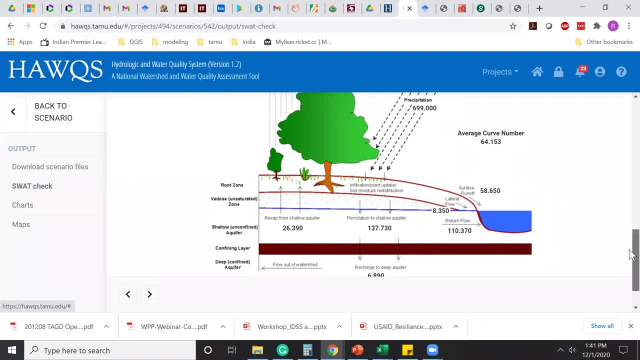 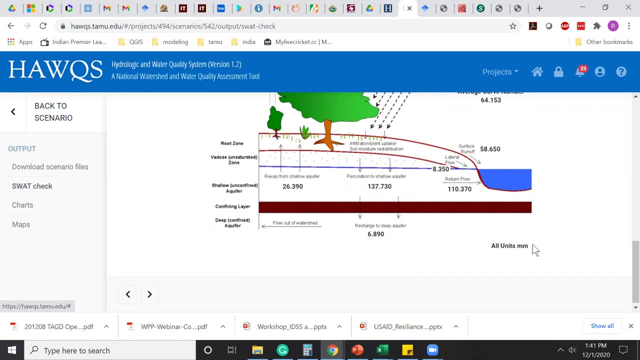 in the watershed is about 64. And this is the runoff: lateral flow, return flow, Return flow back to the river. Okay, You can also change the units. if you are more familiar with the English system, You can change these units actually. 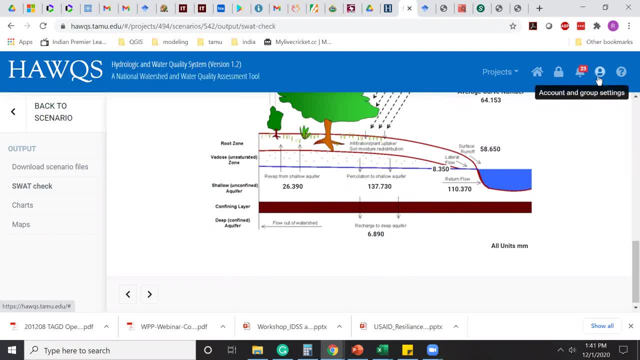 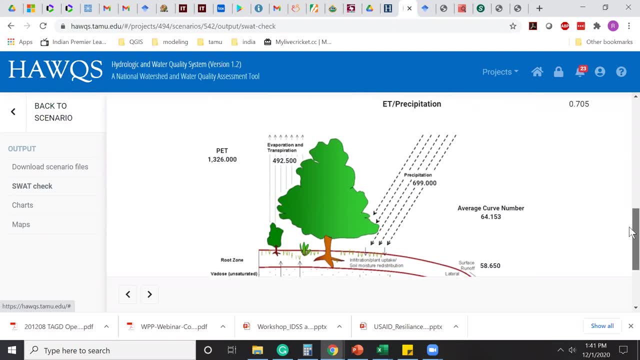 In your user settings, account and group settings. you can go to your account and you say that I want the model. The model will always run on metric system, but you can convert the outputs into an English unit if you are interested in SWAT. 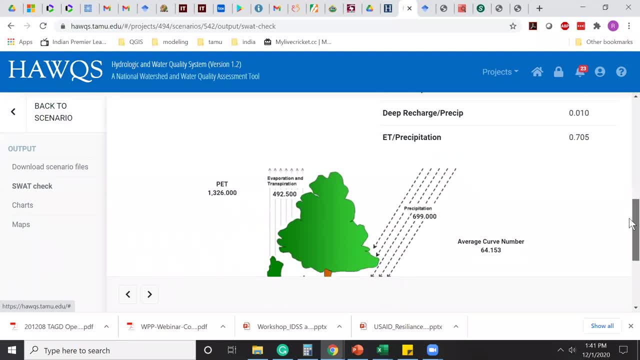 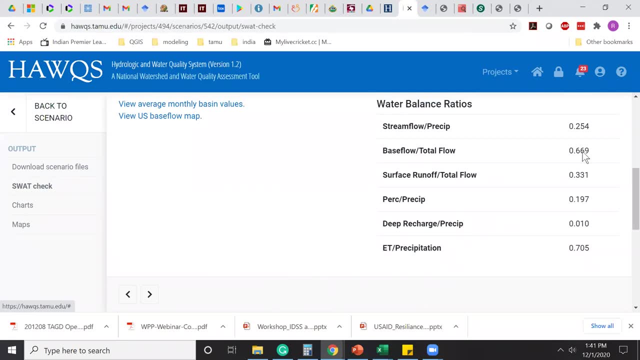 You can see the outputs in English units, more familiar with that than metric system. So this gives you about 70% of your rainfall is 80, but 25.4% is stream flow. Of the 25.4%, 66% is base flow. 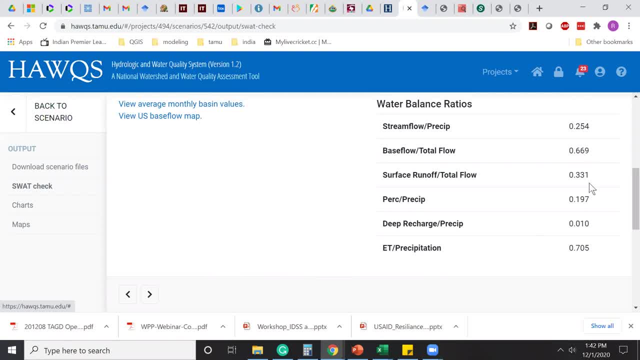 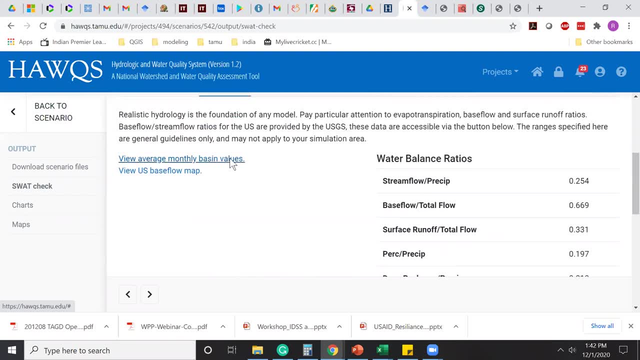 and 33% is the runoff in this watershed. Okay, And if you want to look at the same data on a month by month, you can click on the monthly values. Here is your rainfall distribution for the 11 years on a month by month. 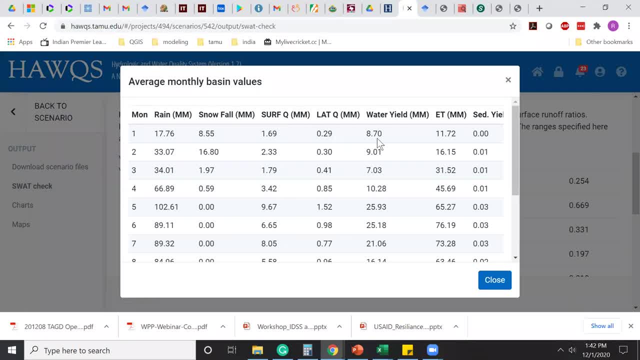 how much was the snow? how much is the runoff? lateral water yield is nothing but your stream flow. These are all expressed in depth, in millimeter, Okay, And sediment yield, nitrogen and so on and so forth, If you are interested. 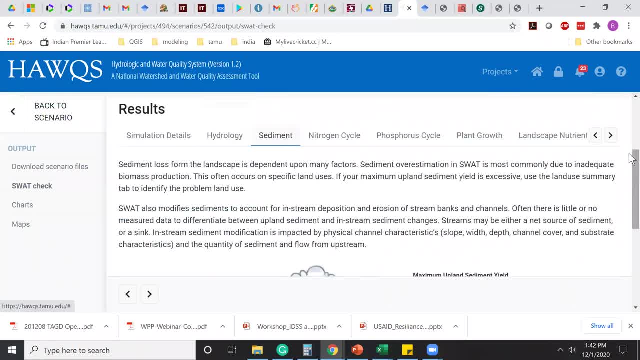 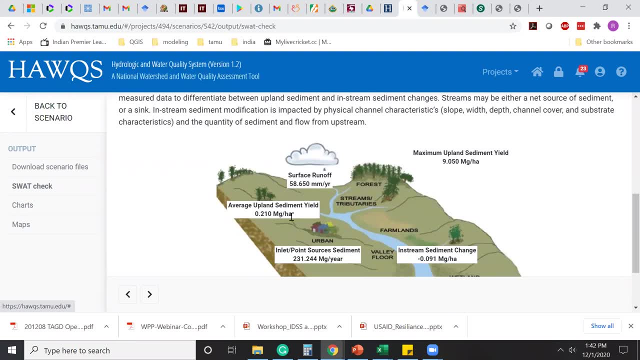 in looking at things like sediment. click on sediment tab. It gives you average annual how much sediment in megagrams means tons per hectare. So it's 0.2 tons per hectare. Okay, And how much is the contribution from the point source? 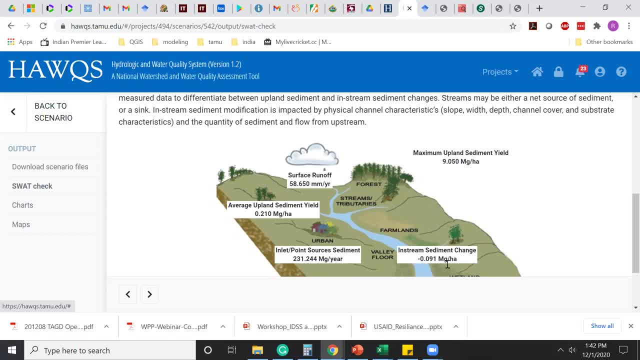 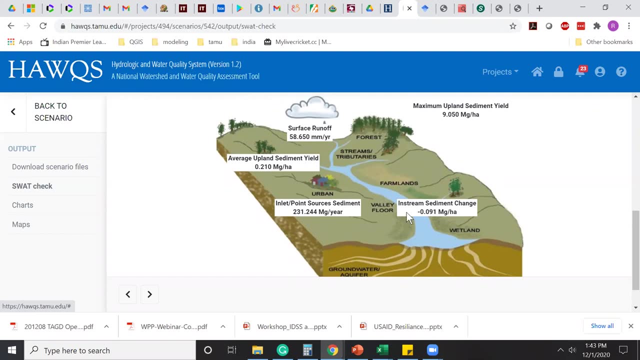 in this watershed And how much of them is either deposited or scouring happening in the channel. When you say negative number, that means you are getting eroded. Your channel is getting eroded. If you get a positive number, your sediment is getting deposited. 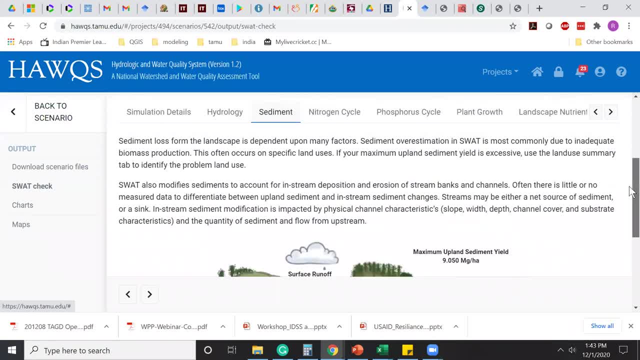 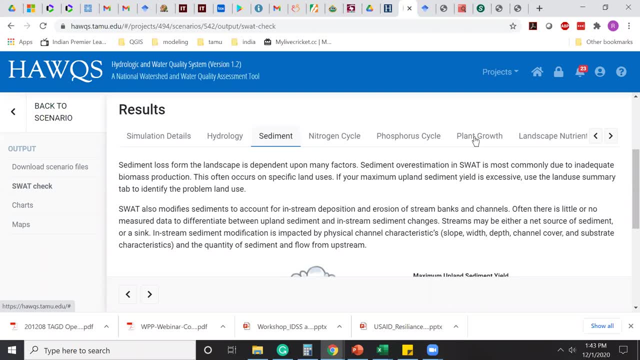 Okay, And you can also look at the nitrogen cycles, phosphorous cycles, plant growth like biomass, crop yield and so on and so forth. Or if you want to look at the losses, let's go and look at it here in the interest of the time. 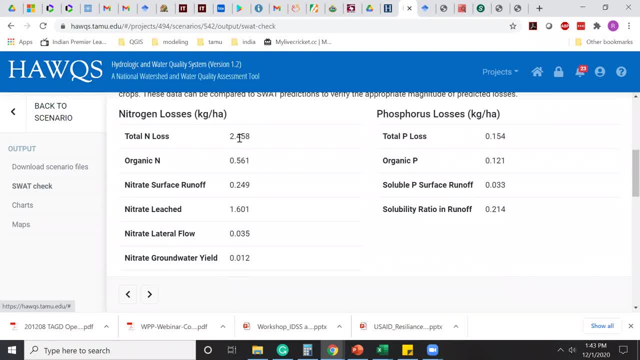 How much is the nitrogen loss, for example, Total loss of nitrogen in the watershed? Of that, how much is the organic nitrogen? How much is the soluble nitrogen? How much is leached to the groundwater? How much has gone through the lateral flow? 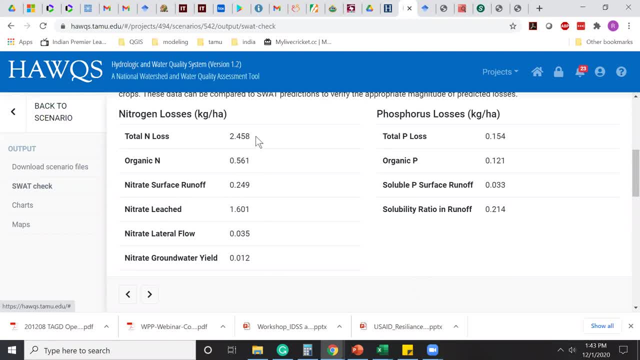 How much is in the groundwater? So you can get the entire configuration. I mean composition of your nitrogen species or nitrogen components in the watershed. This is for all the watershed. Later you'll be able to get the data for a specific HRU. 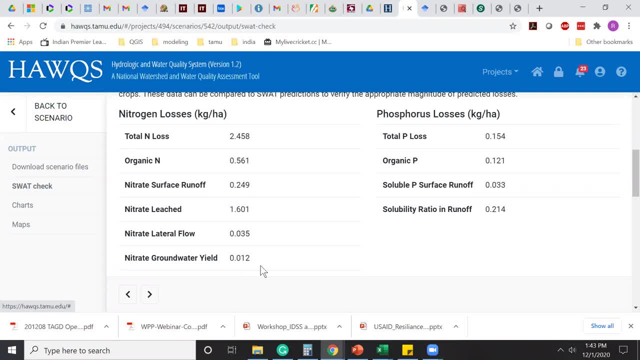 specific land use, specific sub-basin, specific river reach, You'll be able to get the same information. So same thing for phosphorus, Total phosphorus, organic phosphorus, soluble phosphorus and so on, And you can get more detailed information. 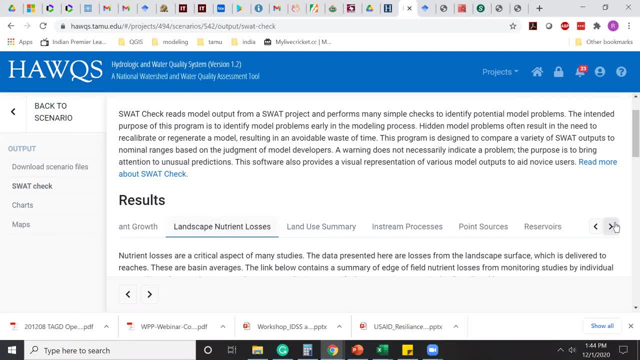 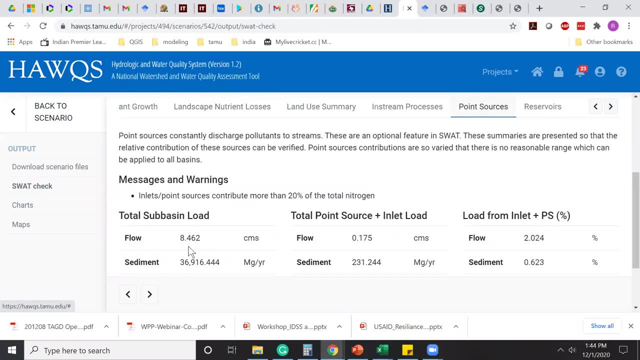 as you can see here, There are more other information like. one of them that may be of interest to you is the point source, for example. So how much is the total flow from the watershed Of that? how much is the point source? 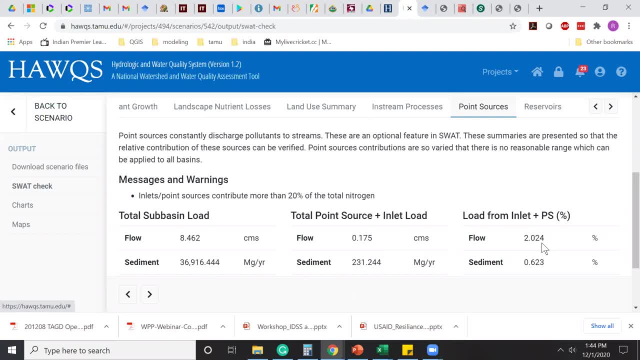 And thereby you can see point source: contributes about 2% of the flow On the sediment. how much tons per year? How much is the point source? There's about 0.6 tons per year. So same thing for nitrogen loss. 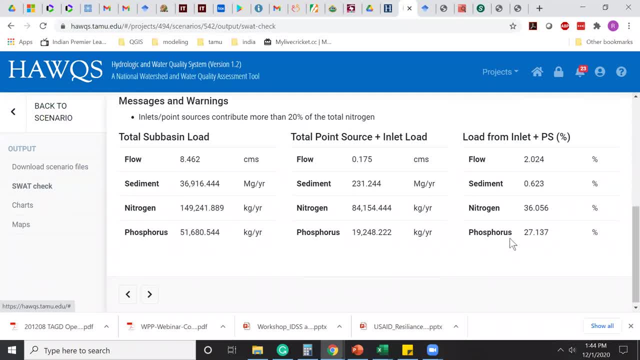 Same thing for nitrogen and phosphorus. So if you're looking at load allocation in a TMDL scenario, this will be useful for you to see what portion is coming from point sources and what portion is coming from non-point source, and so on. 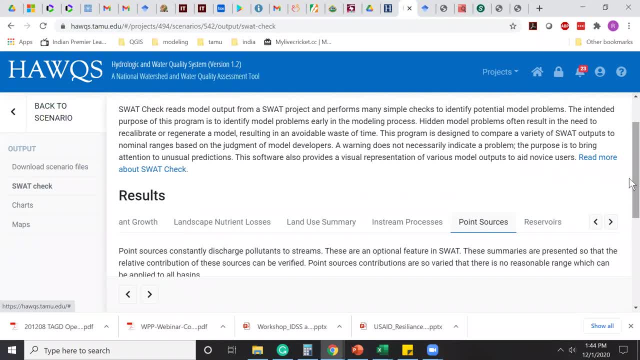 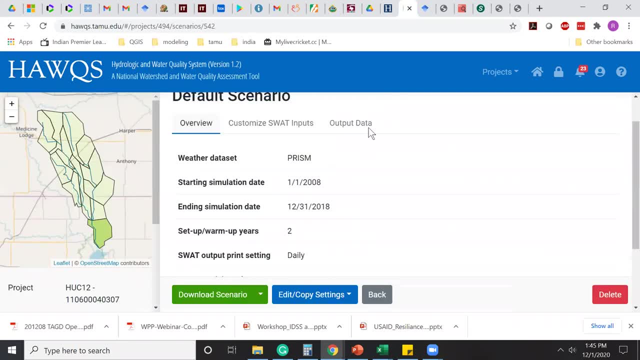 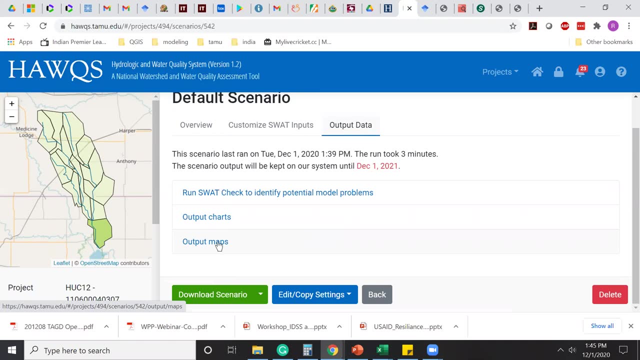 Okay. So let me jump back to show you a few other tools that I wanted to allow you to ask more questions for me, So you can also create maps. Okay, I don't have the time today to show you the competitive chart If you run multiple scenarios. 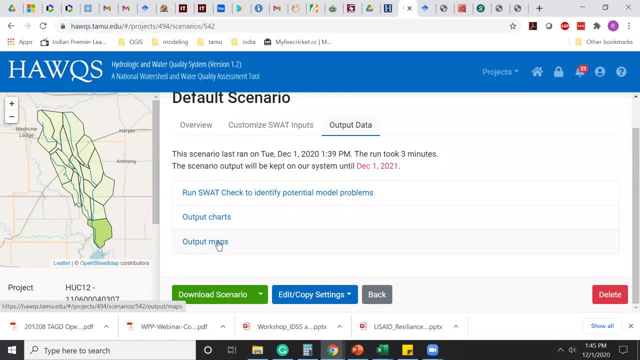 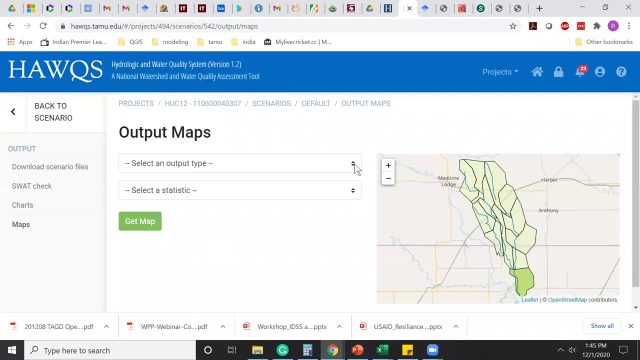 you'll be able to put maps side by side to show them before and after. Okay, Same thing on chart. You can do comparative charts. So let's say I want to show the sub-basin output. What statistics? Let's say I want to look at the average annual. 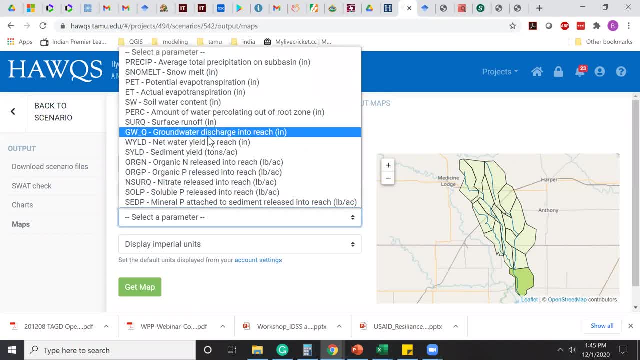 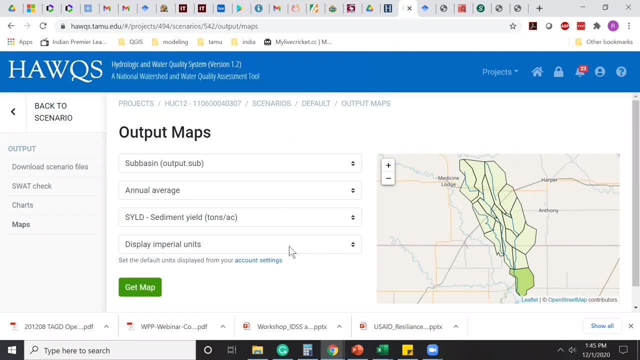 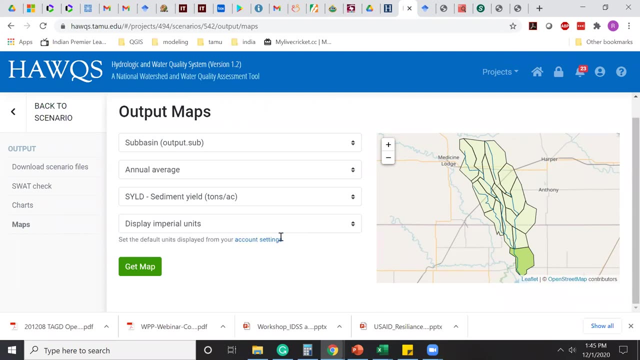 and what parameter you want to plot. Let's say, I want to look at the sediment yield. I mean, I'm just picking out And you can choose whether you want displaying imperial or metric units- Okay, Like English units- or metric units. 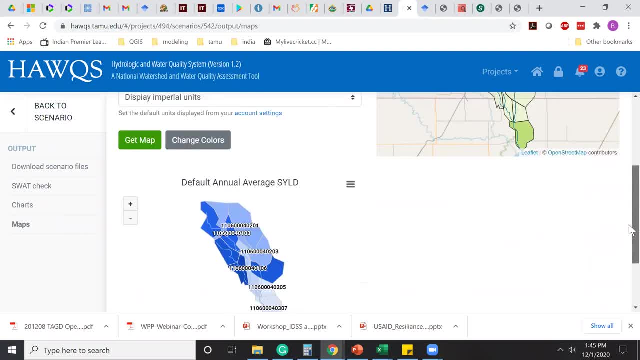 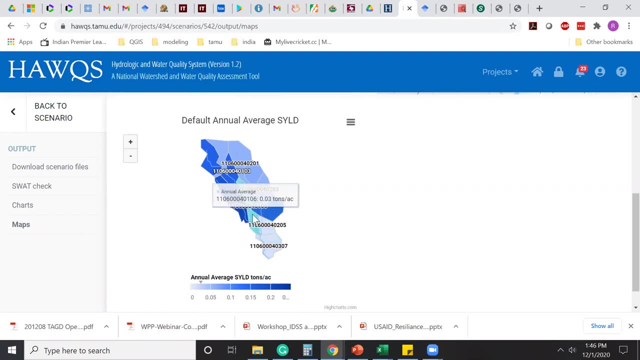 And you say: get me a map So it'll show you how much is the average annual sediment. So here is the scale. So if you move your cursor it'll tell you it's 0.03 tons per acre, It's 0.06 tons per acre. 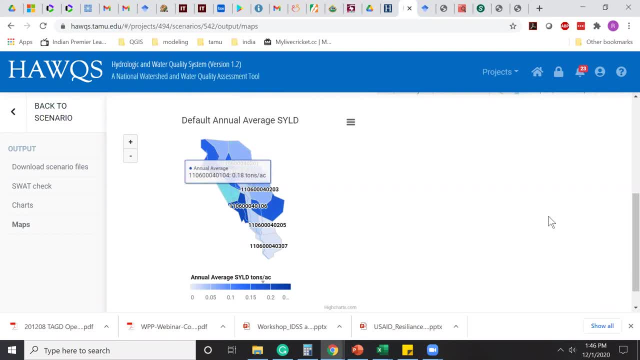 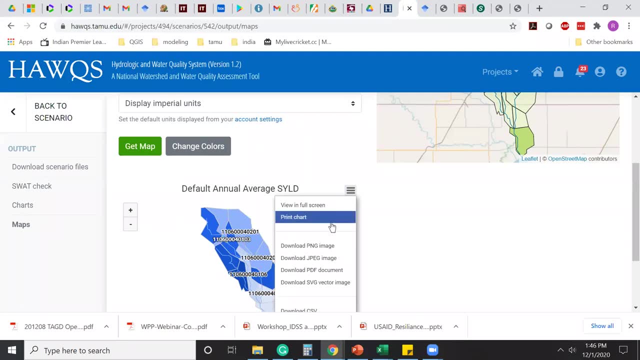 This is 0.18 tons per acre, And so on and so forth. You can change the color. You can just click on this here, change the color. You can export this into PDF And you can print it directly. You can save it as a PNG image. 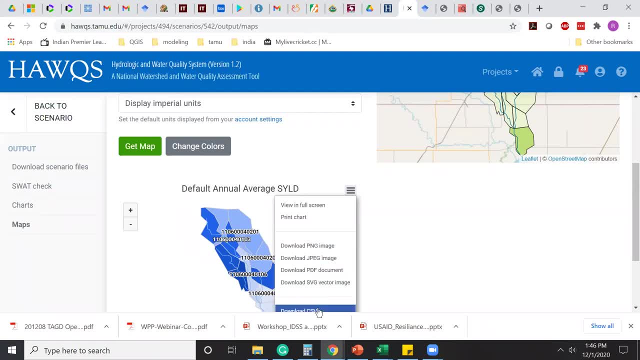 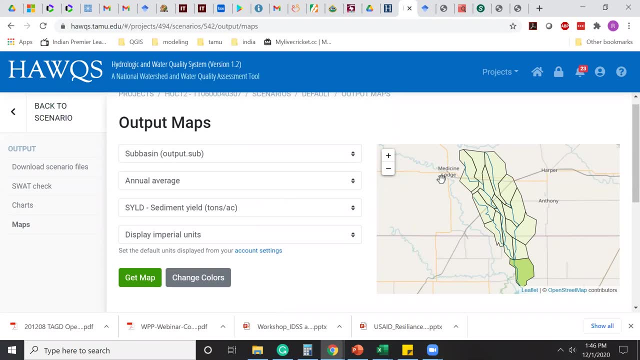 or JPEG image So you can download the data as a comma delimited file. So you have all kinds of options to customize your output in a way you want it actually And you can print them all together. Okay, And if you had the multiple scenarios? 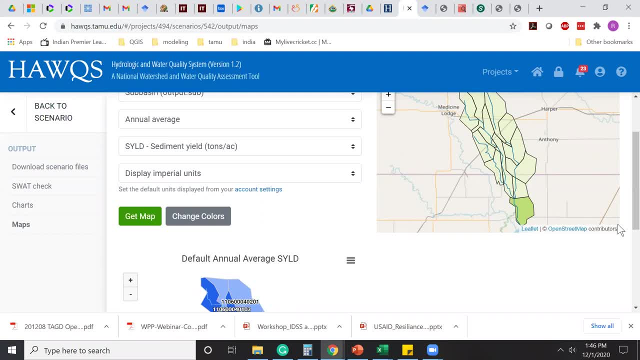 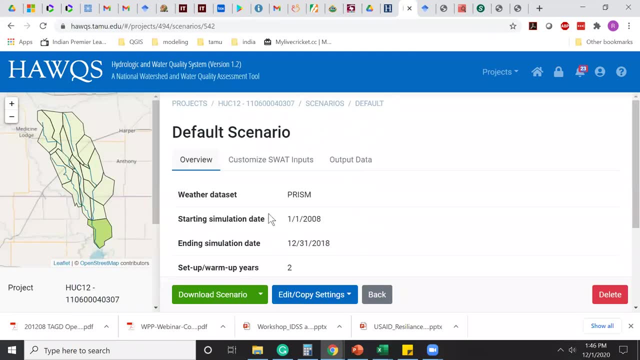 I could have chosen both scenarios and I showed you the map side by side. It'll plot all of those outputs. Or let's say you want to look at the time series data And I want to look at chart And I say what's happening in the river? 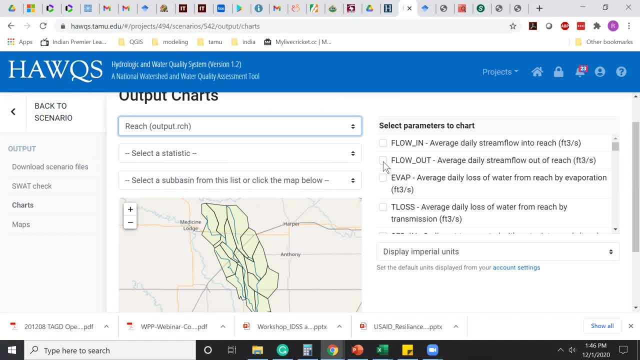 for each output And I say I want to look at the flow And I want to look at, say, sediment, And I want to create as a new axis, add an axis. And if you want to look at total nitrogen, let's say, for example, 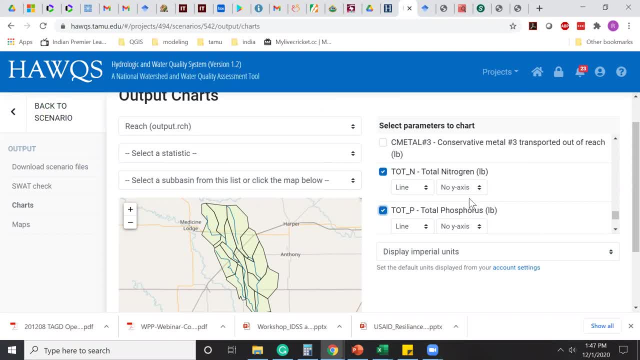 total phosphorus. Again, you can choose your units. I can choose multiple axes. And what statistics? Let's say, I want to look at the monthly. You can also do load duration curve, LDC, flow duration curves. You can do all those stuff here. 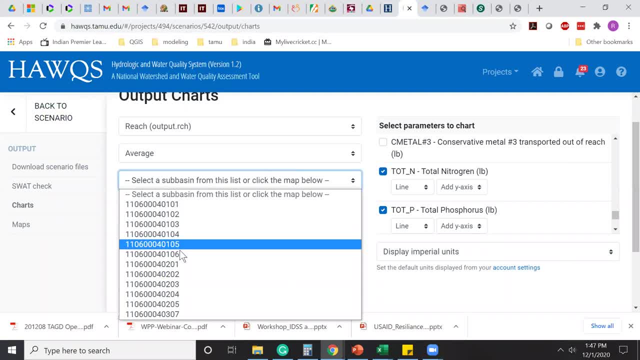 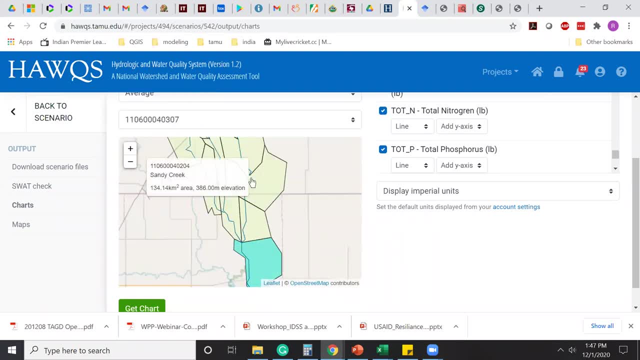 Or box plots. You can select where exactly you want to look at by picking the sub-basin number, or you can just click on the map. Okay, I want to look at the output of the watershed outlet And maybe somewhere in the middle, for example. 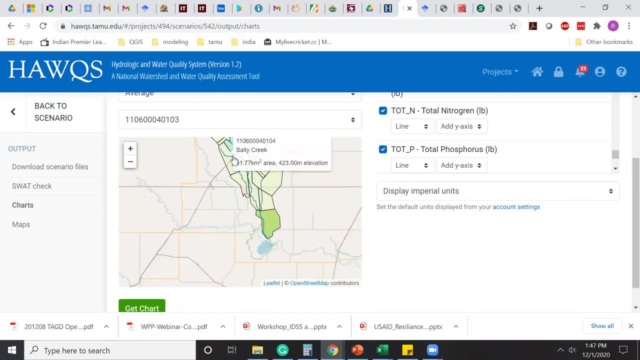 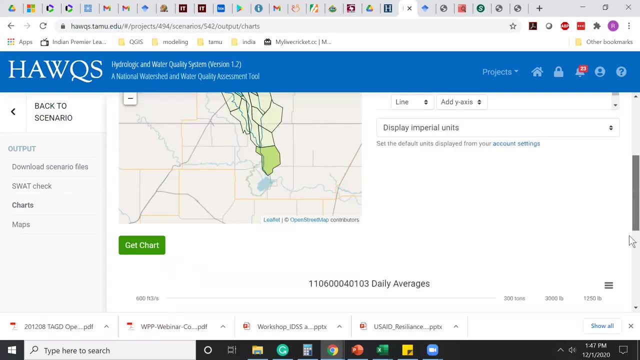 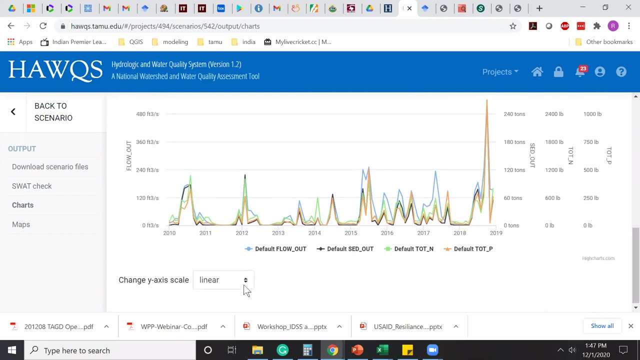 So I also want to look at right here. So I can have multiple locations, I can choose And I can say: get my chart. So here is the value at that location And you can also change your axis from linear scale to log scale and so on. 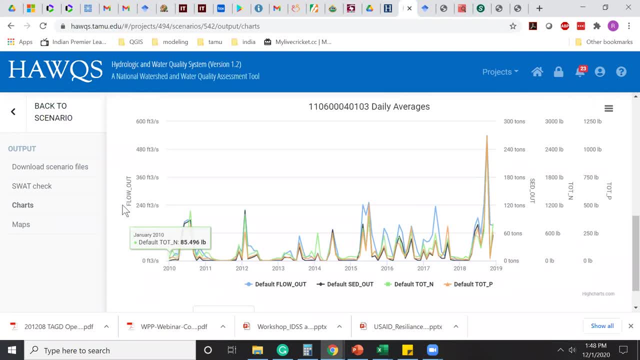 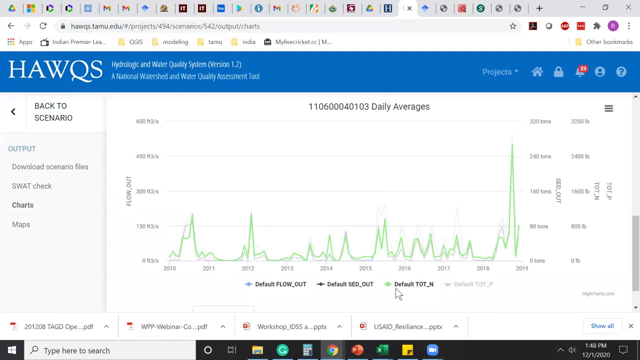 And it shows you the flow in cubic feet per second, because we use the English units and sediment out in English: tons, pounds of nitrogen, pounds of phosphorus. If you don't want any of them, you can just simply click on it to disable that actually. 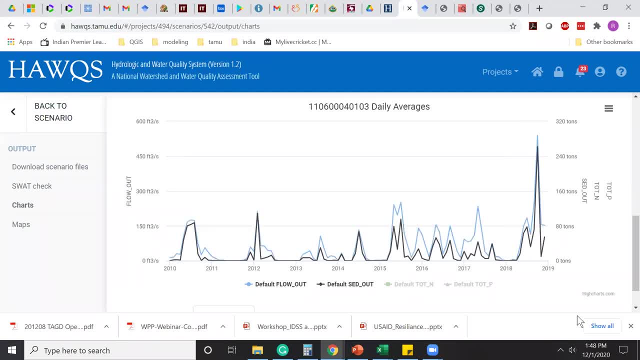 And you go on to look at the flow of nitrogen. You can just look at the flow of nitrogen, for example, And again, you can export this data. You can export this map, You can print it, You can download the image, and so on and so forth. 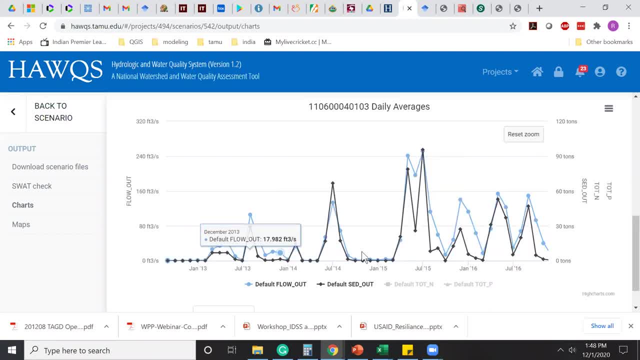 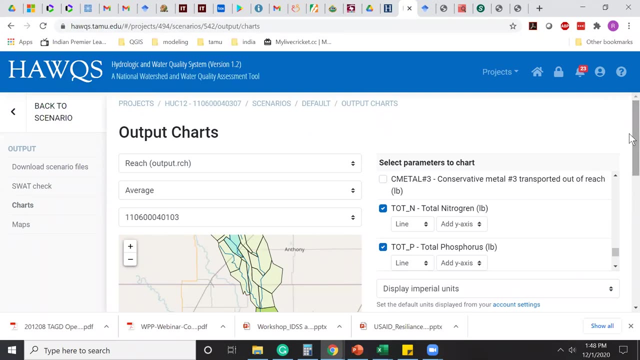 You can also zoom in for a particular thing. You can get into much more detailed output by zooming into the map. So there are lots of features, not only to build a model, visualize, analyze and compare different scenarios, and so on and so forth. actually, 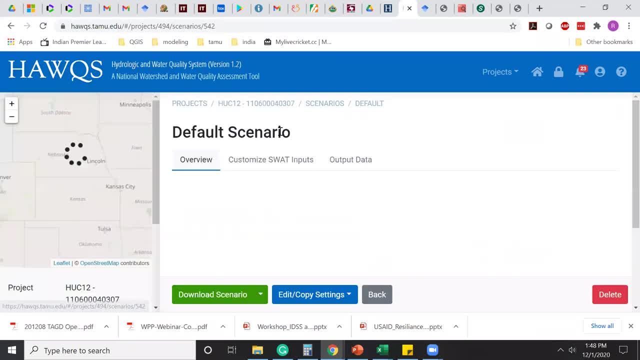 In the interest of the time, let me stop right here and maybe answer more questions, And I'm sure later you're planning on doing a more detailed workshop That'll help you. But also you can play around with the tool as time permits in the meantime. 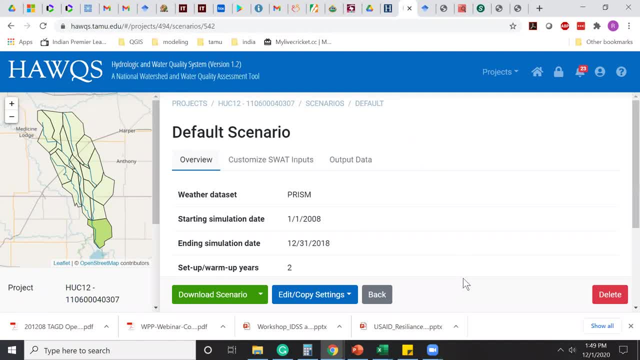 Kevin, is it a good time to stop myself and maybe I'm allowed to answer questions? Sure, I see you've already got another question in the chat. Export table of input data used in the analysis, for example, time series of total phosphorus. 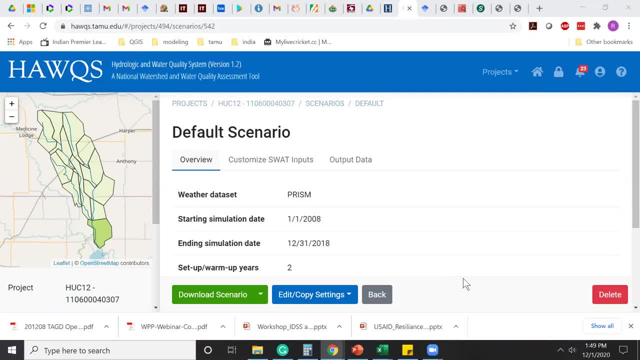 Absolutely. yes, You can do that very easily. The plot that I showed you. you can pick and choose anywhere in the watershed and say: plot that map. While it's plotting the map, you can also ask to export that map or export that plot or export the actual data. 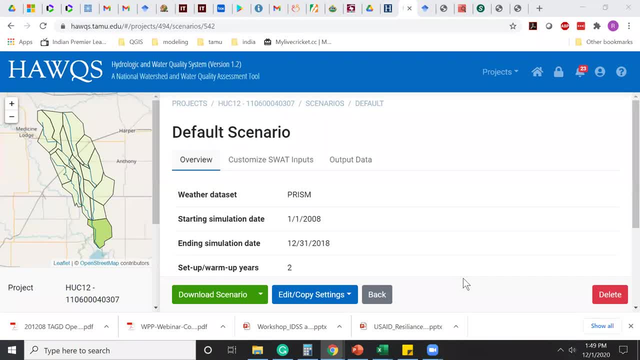 that's coming off of the modeling system. Yes, you can do that. So, Srini, I've got a question. So, dealing with future climate scenarios, is this tool equipped to bring in some of those as well, or do you have to do this? 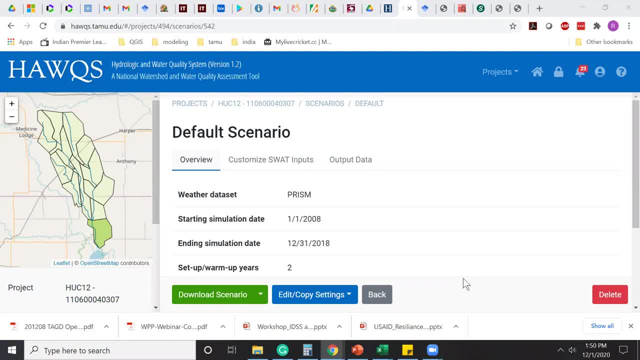 or you have to do that offline. Currently, the national database available for climate change models are only at the level of eight and 10 digit watersheds, not at the 12 digit, In other words, downscaling to a 12 digit. 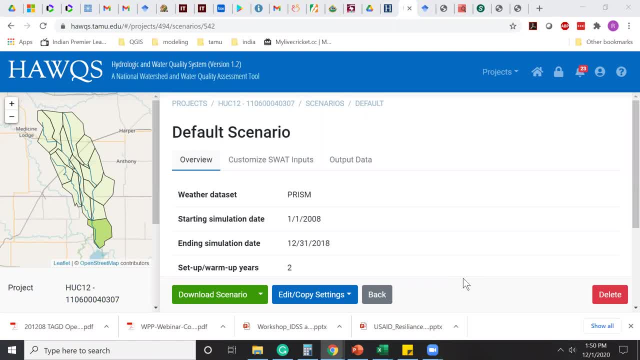 is not advisable yet because of the uncertainty it poses actually. So what we could do is- I do have about 12 models that has been already downscaled and projected for the next 100 years with different scenarios: RCP scenarios 4.6,, 2.6 and say 8.0. 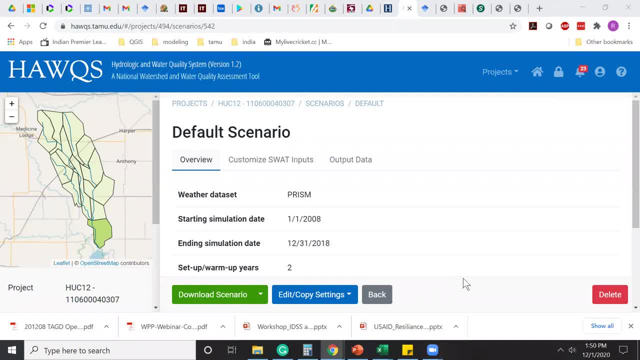 and so on and so forth. 8.5.. So we can take those models. they are applicable at the HUC-12, sorry, HUC-10 level, but we can apply to the same to all the HUC-12 within the HUC-10, for example: 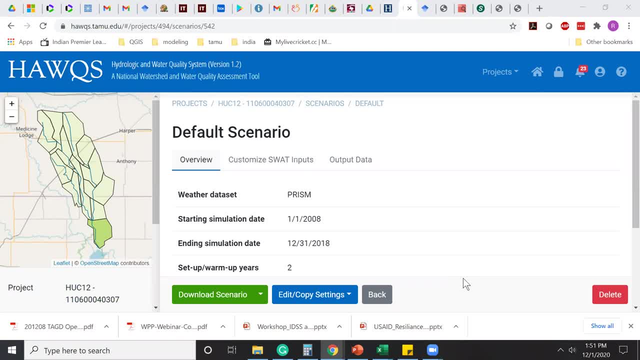 and you're able to run the model. So that feature is already available and we could certainly that data is already available. We can try to bring that in here and make that as one of the scenario feature that user can choose to run climate change scenarios and so on. 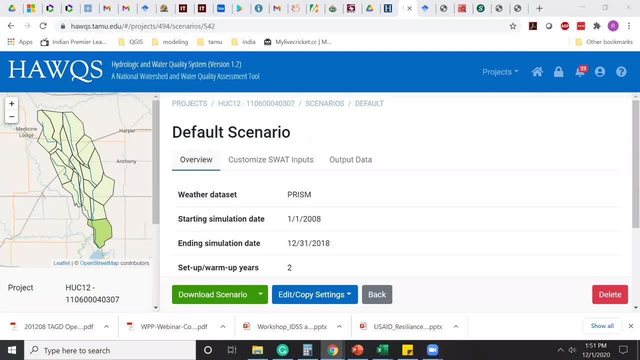 Okay, Can the user. one other question online is: can the user augment the input data with their own data? Yes, it's on a limited basis, For example, with the online data, if you, if you take the whole model offline. 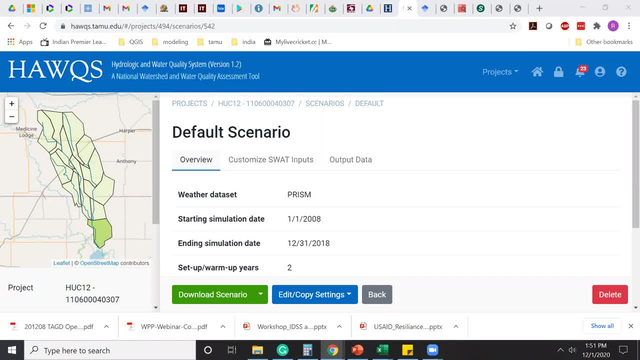 and do it on your desktop, then you have nth degree of customization. You can change any inputs, you can add your own inputs, and so on. However, if you are going to add your data onto the existing online system, we can update land use change. 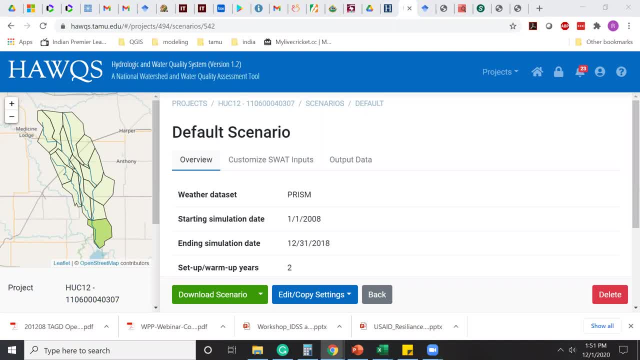 we can update weather input, we can update point source input, for example, and you can- obviously you can- change land management and so on and so forth. So I need to know a little bit more specific exactly the type of input that you're thinking. 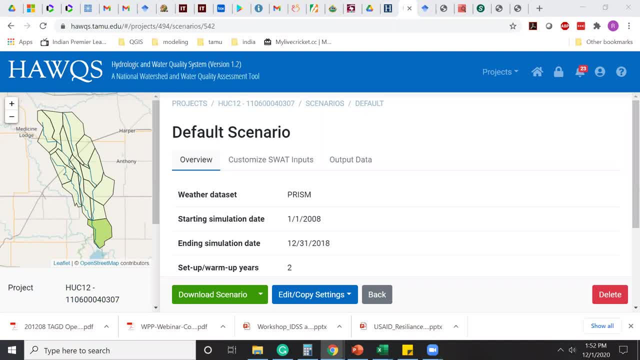 whether that's allowed or not actually, but right now we have a limited set of user input that can be updated as part of running scenarios. Any other questions, comments, feedback. You can unmute and talk also. actually, You don't have to type on the chat box. 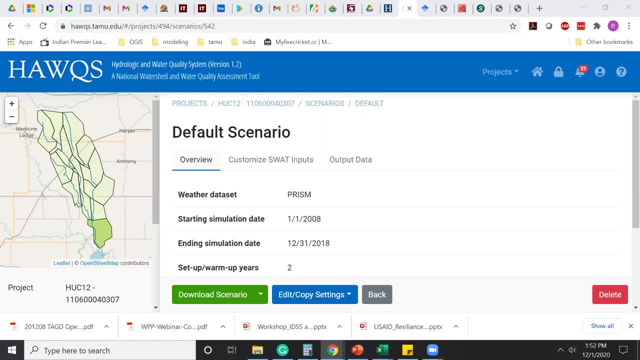 if you want to ask questions. Well, if there are any other questions, definitely feel free to contact us and let us know. So the timeframe for getting the Oklahoma hawks online and ready to use should be late this spring, certainly before the end of May. 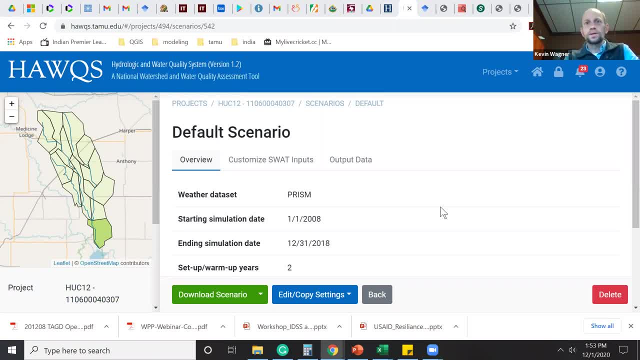 And, like Dr Srinivasan said, we plan to have a one day training session sometime before the end of May as well. So once the tool is up and ready to go, we'll be having a training to go through each component of the hawks model. 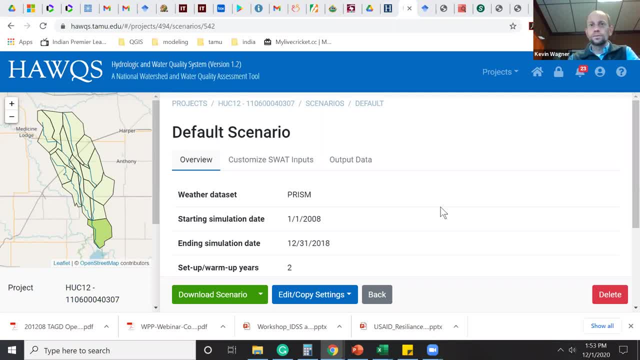 and allow you, as users, to give it a try on a test watershed and just to get a better idea of its capabilities and ask the questions that you might have. But, as you can see, it's very much user friendly, especially compared to SWAT. 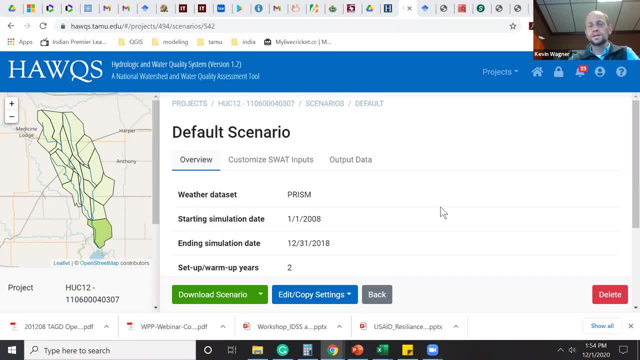 So I think it's pretty exciting to have access to this tool and to have this tool calibrated for Oklahoma. Are there any other questions out there or comments? Well, if not, we really appreciate your participation today, Dr Srinivasan.